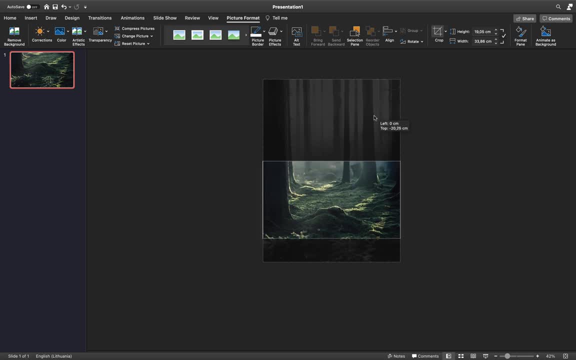 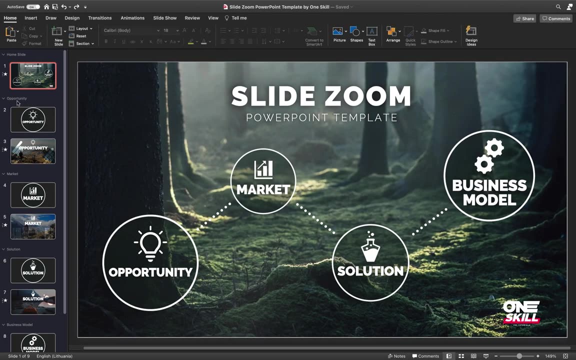 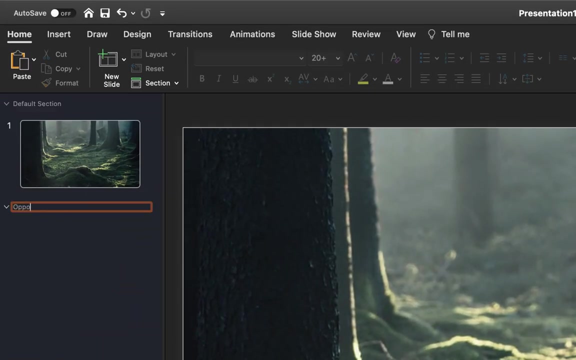 to the size of our slide and at the same time, you can adjust the positioning of your photo inside of the crop area. that's awesome, all right. so next we have to add our first slide section. so let's just right click and choose add section. let's give it a name, for example, opportunity. that's awesome. let's insert a blank slide. 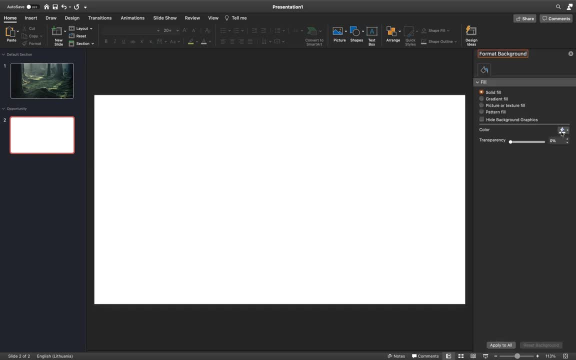 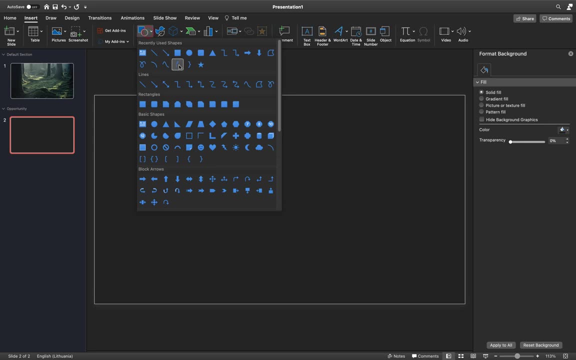 and let's give it a dark background because we will be inserting some white circles. so this way it will be easier to work. now let's just go to insert shapes and let's choose this circle shape, hold down the shift key to get a perfect circle. that's awesome. we can activate the 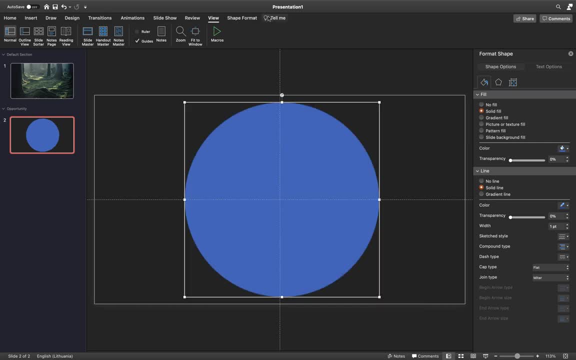 slide guides so that we can see where's the center of the slide. and now let's just align that circle to the middle, into the center of the slide, and let's make sure that our circle has a white outline, and for the width we can insert 10 points. that should be fine, and 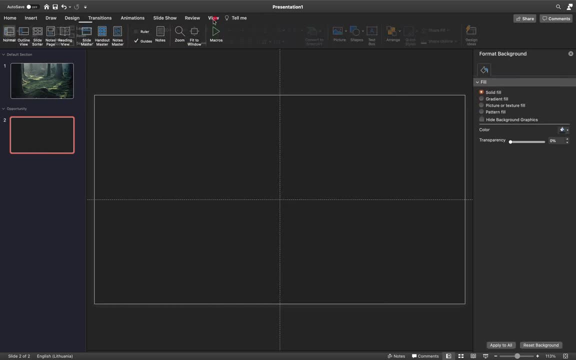 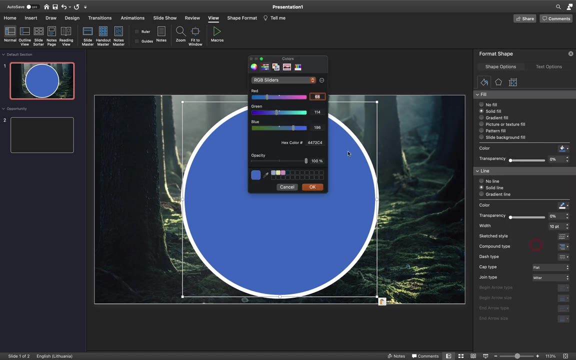 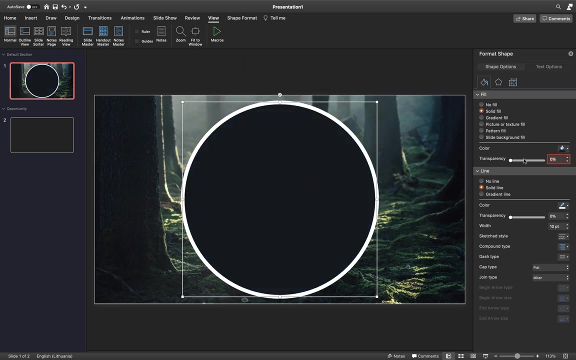 now let's just cut this circle and let's paste it to slide number one, because here we will just use the eyedropper tool and we will copy this beautiful color from the tree from the first slide. I think it looks nice to use the same colors and let's just add some transparency to our circle fill, that's. 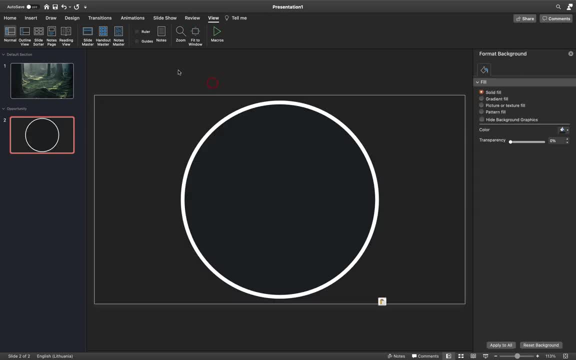 awesome, and let's cut and paste it back to slide number two. that's wonderful. alright, ladies and gentlemen. and now let's just insert a text box. now you cannot see anything because the text is in black, so let me change it to white column, alright? so this is our text box opportunity, and let me actually go to my 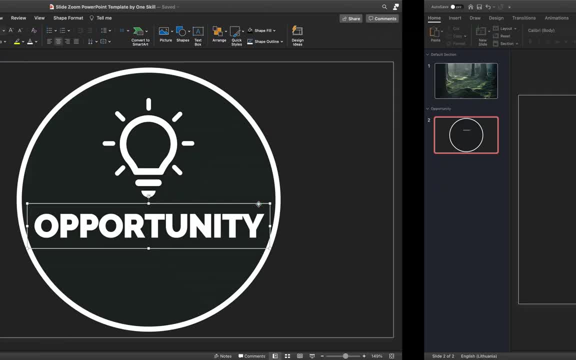 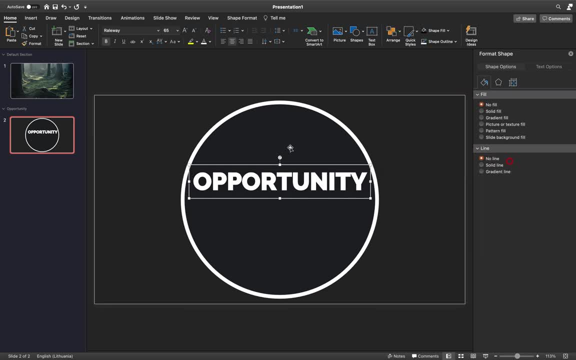 previous presentation and copy the style of this text box and let's just paste the style to this text box. this way, we can save some time and let's make sure that the text box is in the center of the slide. that's awesome. right and next, as you can see, we 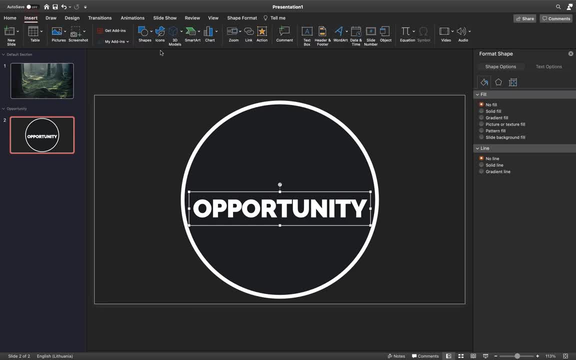 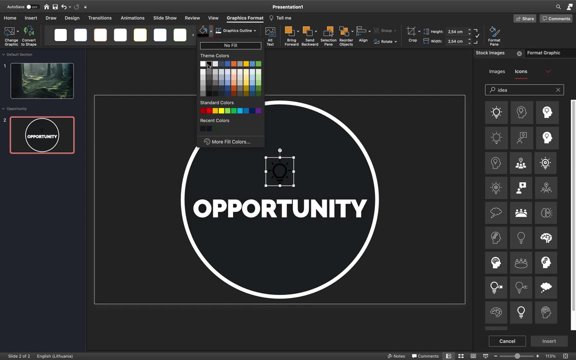 need to insert this light bulb icon, so let's just go to insert icons. if you don't have icon tab on your PowerPoint version, you can always go to websites such as flat iconcom and find icons there, so let's just insert this icon, which is called idea. let's make it white. 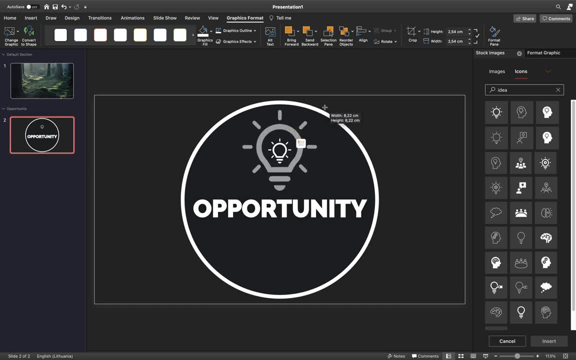 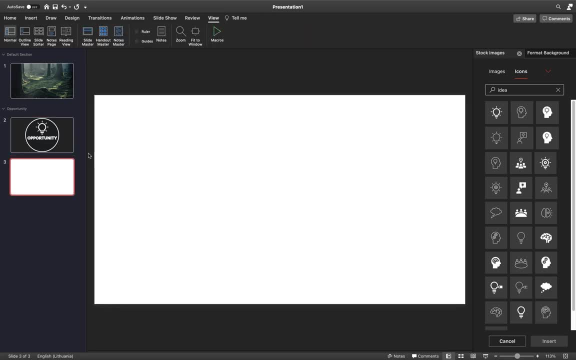 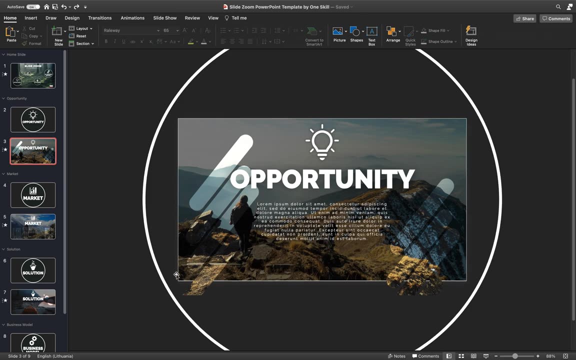 right, and let's just increase its size so that we can see it better. alright, so let's insert one more slide, and now we will have to create this opportunity slide. so, as you can see, we have light bulb, we have opportunity, text box and we have this huge circle, so we can basically copy all of these shapes from. 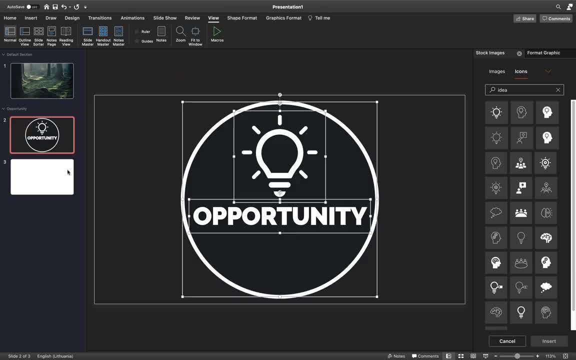 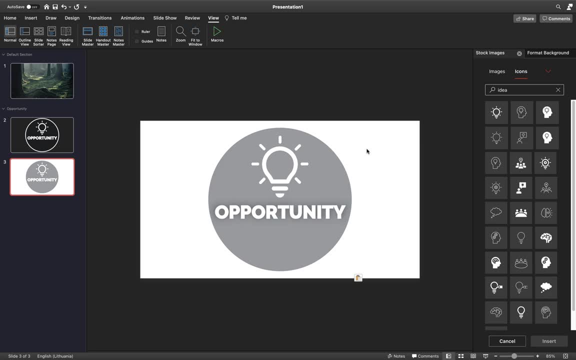 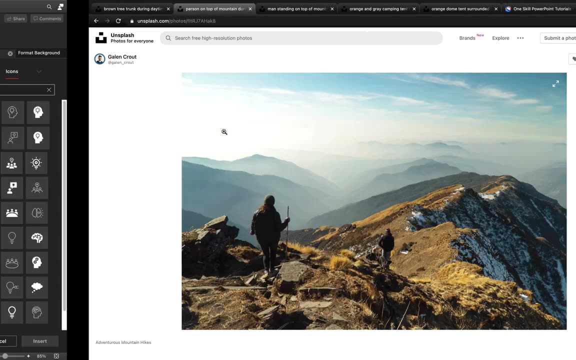 slide number two and let's paste them into slide number three and, as you can see, our slide background is completely white. so let's just find another beautiful picture from Unsplashcom we can use. let's hit copy. and now let's just go to format background and let's choose. 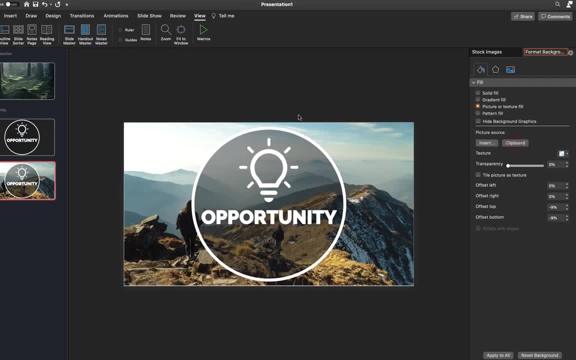 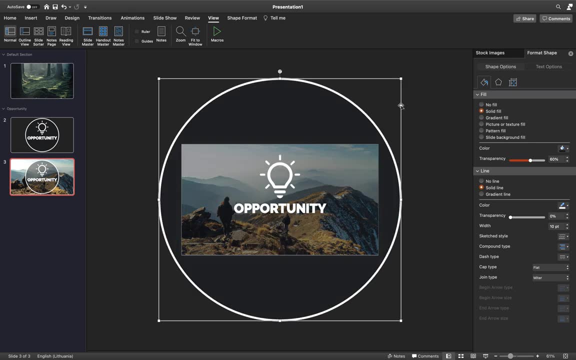 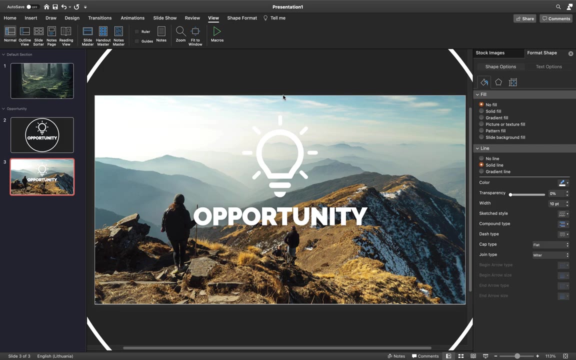 picture and clipboard, and this way we have successfully pasted that picture as our slide background. alright, now let's grab the circle and let's increase its size so that it goes outside of the slide. let's make sure it has no fill. that's awesome. and now let's copy this image. one more time. So we did that and we're done, so let's save this image. So that's it for this one video. So this is the last one I covered Here. we have a원 flow борУк сирп сирпeterverу бур. 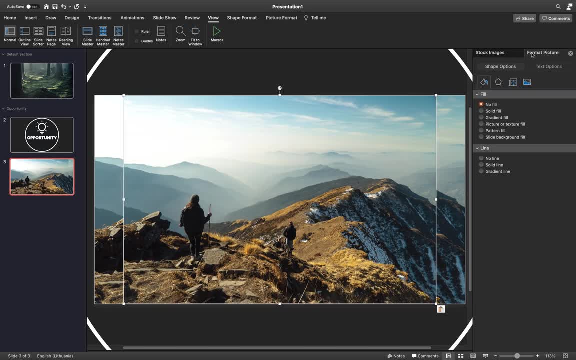 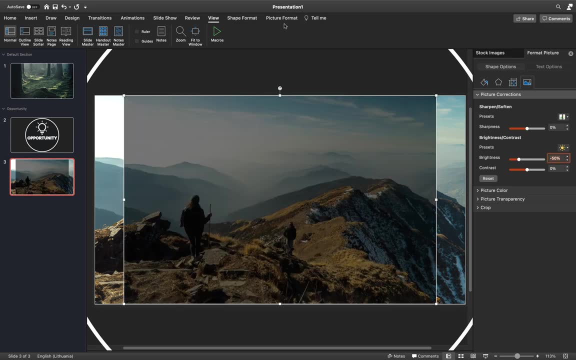 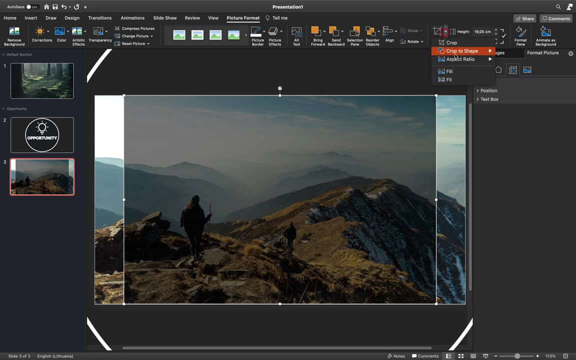 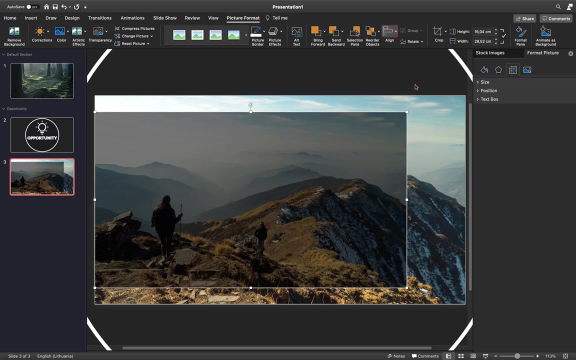 and let's paste it into the slide just like that. and let's go to brightness options and let's reduce the brightness of this image minus 50. all right, let's crop it to aspect ratio. aspect ratio: 16 to 9.. that's wonderful. now let's just make sure that this dark picture covers the 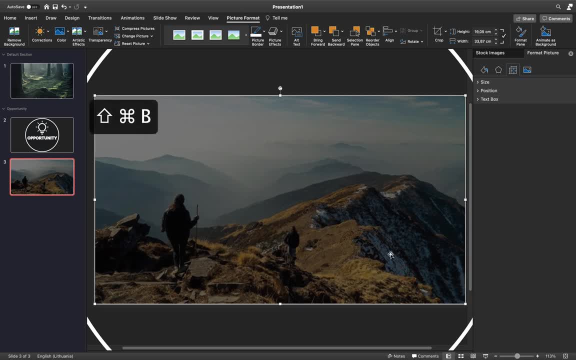 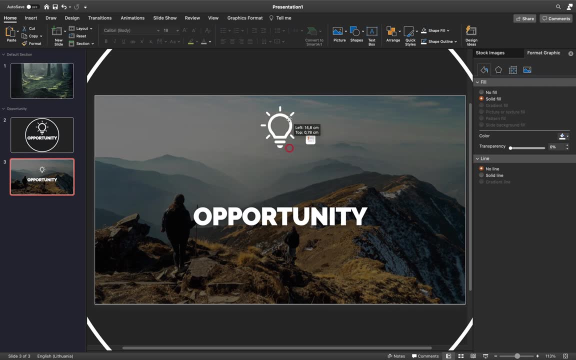 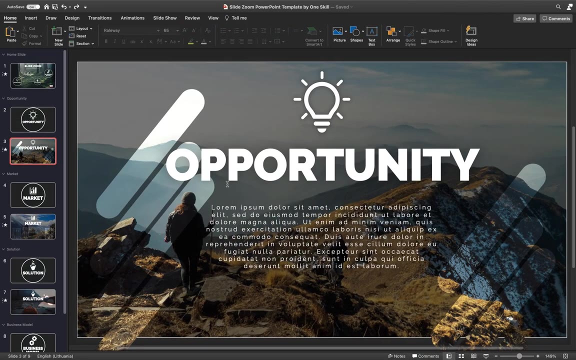 whole slide. don't worry if you don't understand this step. soon you will see why we're doing this dark picture. all right, and now let's continue working with the rest of the shapes. so let's reduce the size of this light bulb and let's increase the size of the opportunity text box. 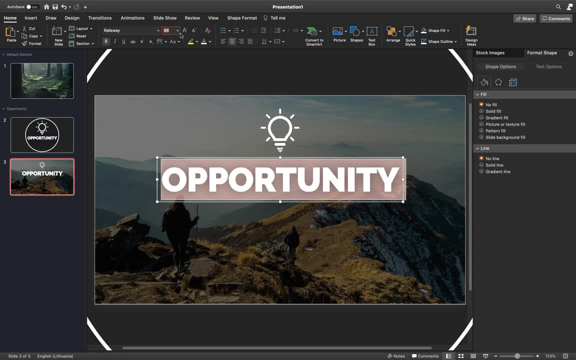 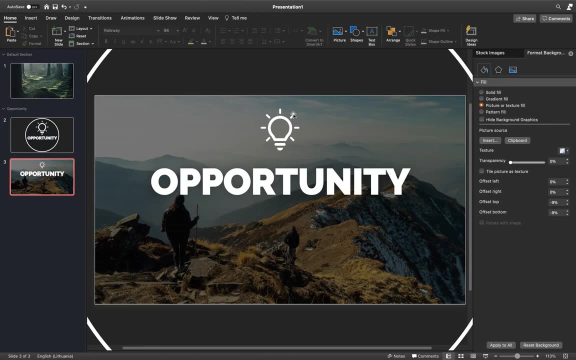 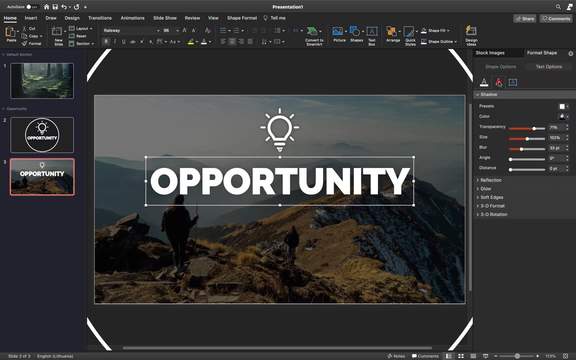 so let's give it a font of 88. you can make it even bigger, just like that. and let me just copy the shadow of this light bulb. let's paste it here to this one. that's awesome. and let's make sure that our opportunity text box has some shadow as well. all right, you can always play with the transparency blur. 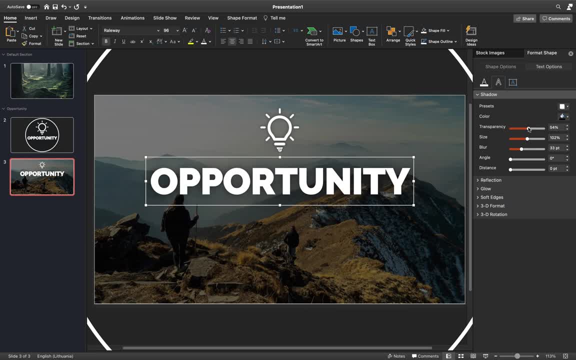 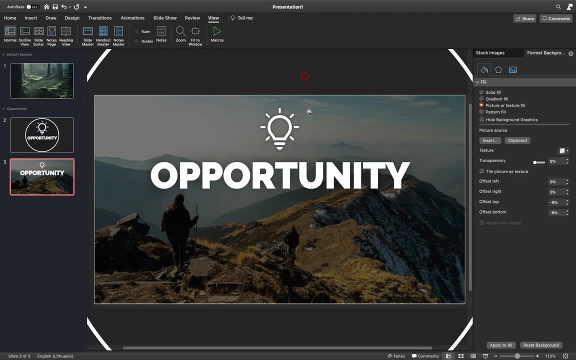 and size to get any look that you want. that's beautiful. and now let me just copy this text from my previous presentation to save some time. all right now, a really important step: we have to set a more advanced physiognomy structure. come back to theellenomnisecom. all right now, a really important step. we have to set a more advanced physiognomy structure. come back to theellenomnisecom. a more advanced physiognomy structure. come back to theellenomnisecom. all right, now, let's make it even bigger. just copy the expository central text tail toキرplicate the pixel in the background. 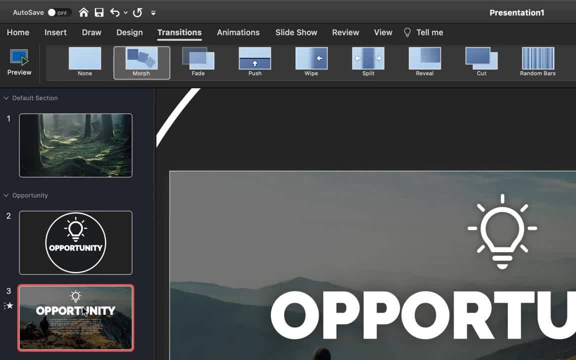 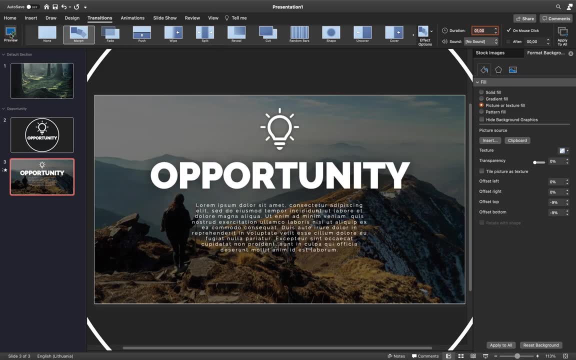 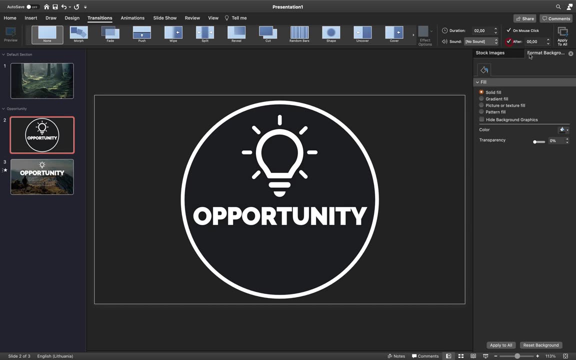 morph transition for slide number three. so let's just go to transitions and choose morph. morph transition will help us to do the animation from slide number two to slide number three. that's awesome. and for slide number two, let's set it to transition automatically after zero seconds. 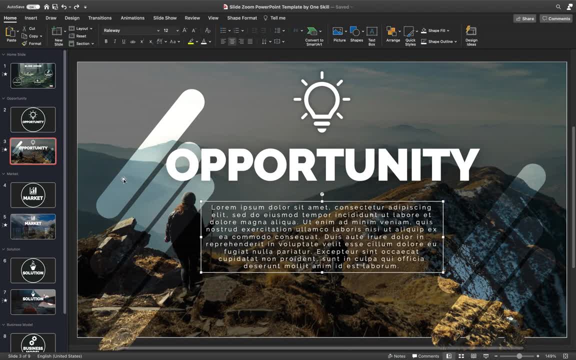 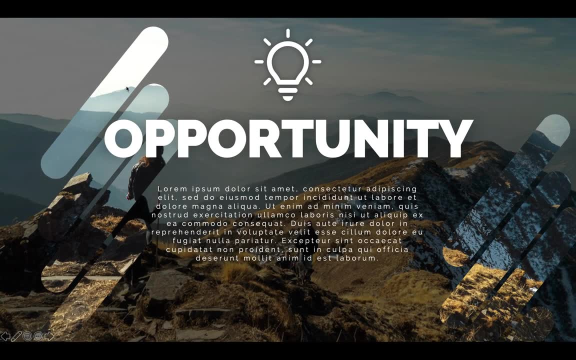 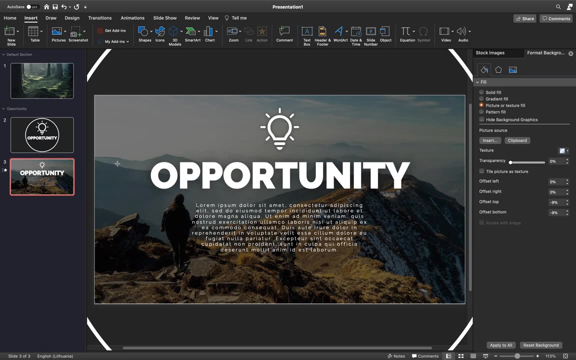 so this will give us a nice, beautiful animation. all right, so now let me show you how we can add these fun looking animated rounded rectangles to our slide. so let's just go to insert shapes and choose rounded rectangle. draw any size and shape that you like. let's make it fully rounded. that's awesome. let's choose no line and for the fill, 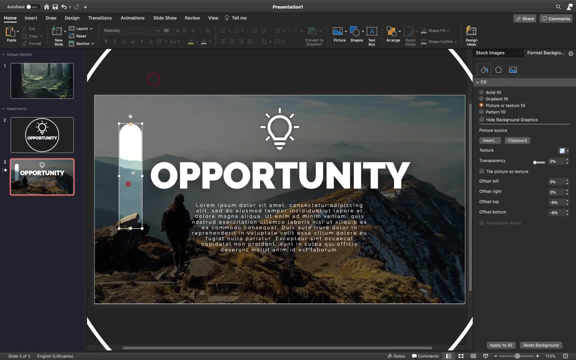 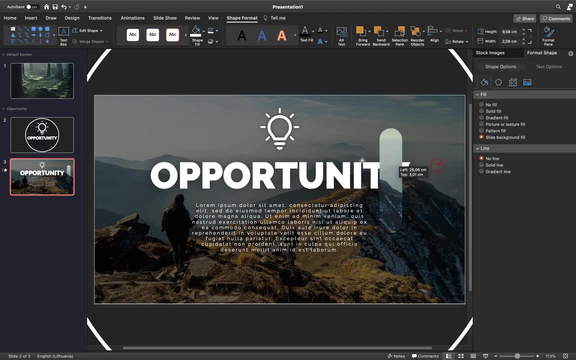 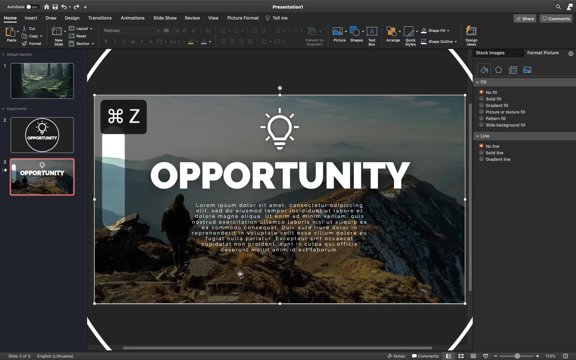 let's choose slight background fill and now, as you can see, this rounded rectangle takes our bright, slight background fill and we're ready for our slide background. as you remember, first we have inserted this bright slide background photo and on top of that slide background we have inserted this dark 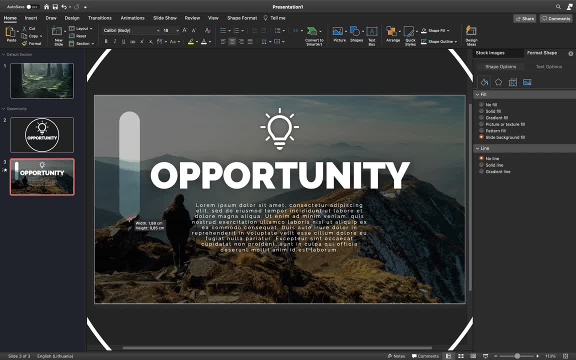 version of the photo and this way we are getting this beautiful effect, this beautiful fill effect, for our rounded rectangle. that's awesome. so now we can rotate our rounded rectangle, just for fun, and let's just place it anywhere that we want, for example, to the right side of the slide, and let's just make. 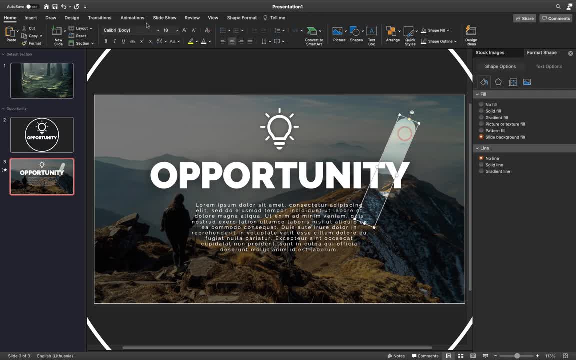 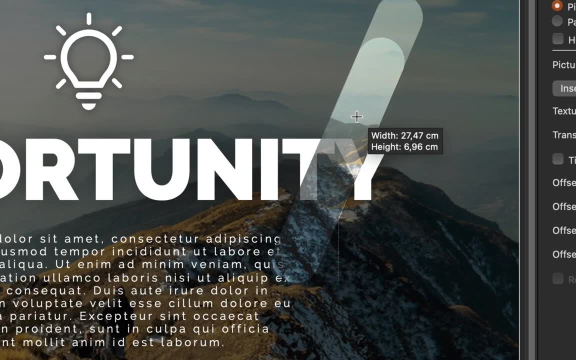 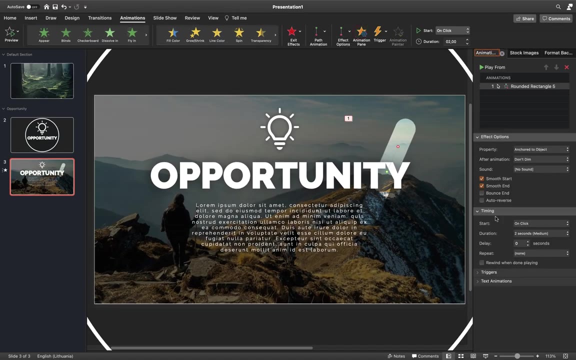 sure that our text boxes stay on top. that's awesome. now we can go to animations, path animations, and let's choose line. now let's grab this red bubble and let's make sure it goes upwards, just like that. that's awesome. and now, in the animation options, let's make sure that this animation auto. 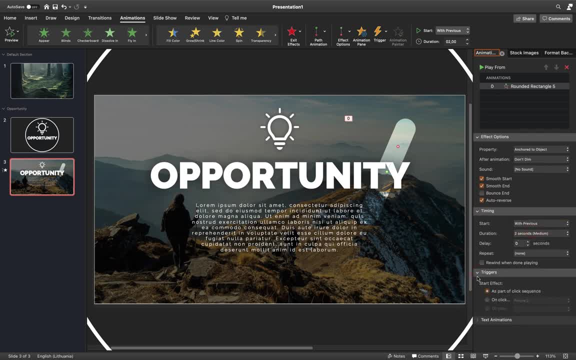 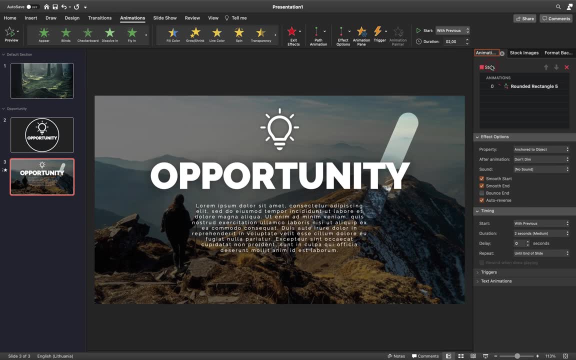 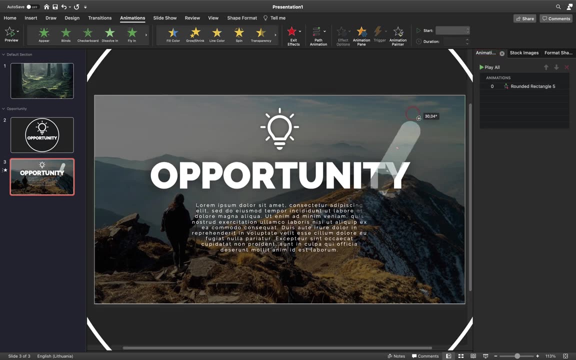 reverses, it starts with previous and that it repeats until off slide until the end of slide. okay, and for the animation duration I'm using two seconds so we can rotate it a little bit more. adjust the red bubble as well. right now we can make some quick copies. you can hold down option on Mac or. 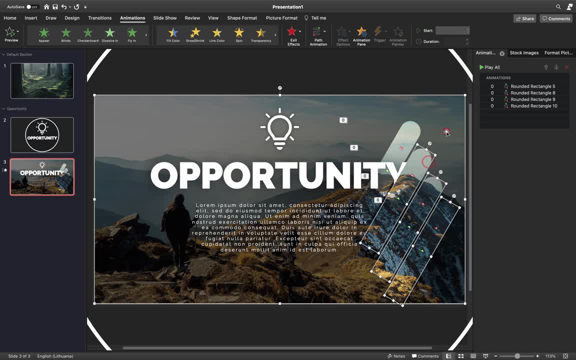 control on Windows and let's make sure that our text boxes stay on top. now let me add a little bit of delay for each of these rounded rectangle. so 0.4 seconds for this one, for the third one 0.8 and for the last one want 1.2 seconds, and we 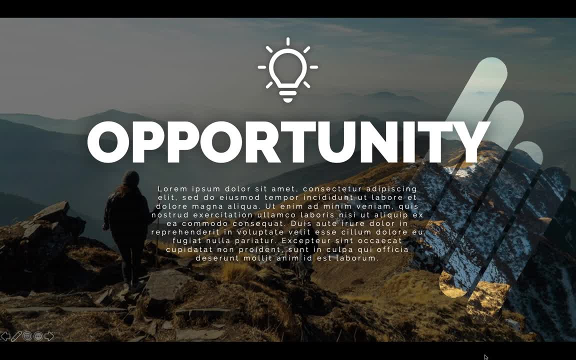 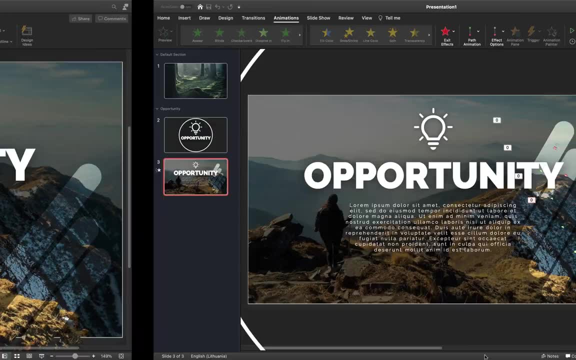 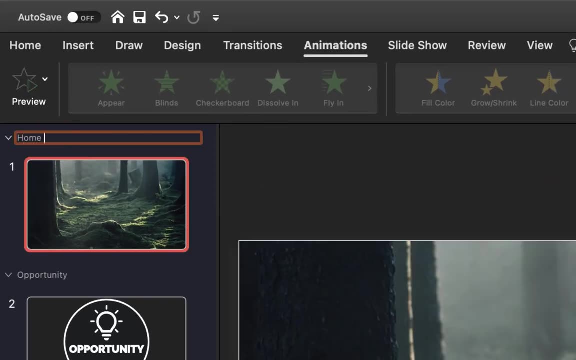 should be getting this beautiful animation of rounded rectangles which are using slide background as their fill. that's awesome. all right, so now we can start inserting some section zooms. before that, let me just rename our first section to home slide. that's beautiful, and now let's just go to insert zoom and 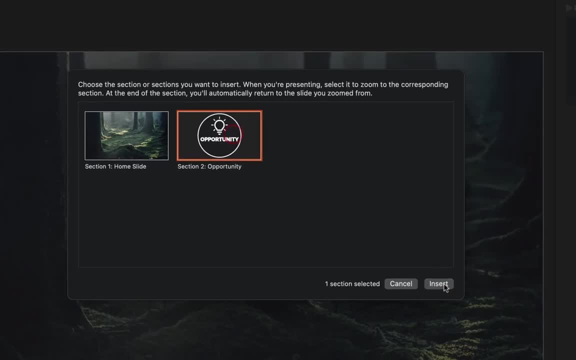 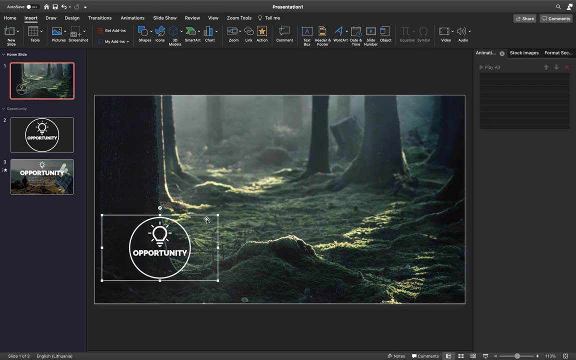 choose section zoom, our first section opportunity. let's insert it and let's right click and choose zoom background. this makes our section zoom background transparent. that's awesome. let's position this section zoom anywhere that we want. that's beautiful, right. and, as you can see, this section zoom covers. 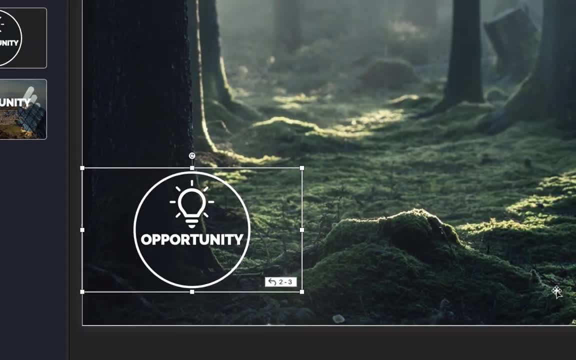 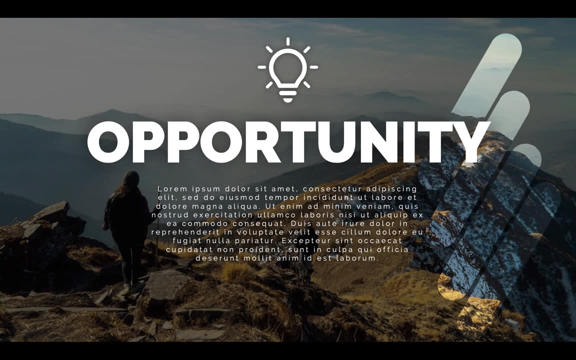 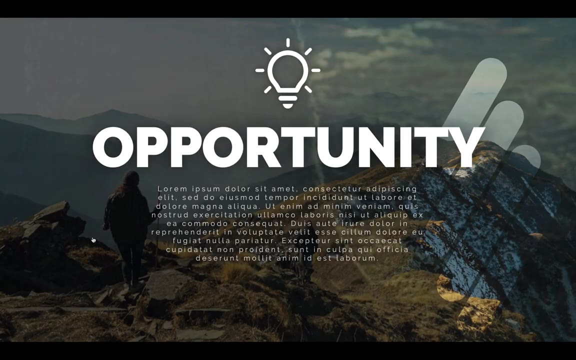 slides from two to three and then it goes back. that's awesome. so I guess we can check it out on full screen. we click on the section zoom and we automatically transition to this last slide in the section and when we click, we zoom back. easy peasy, lemon squeezy. alright, ladies and 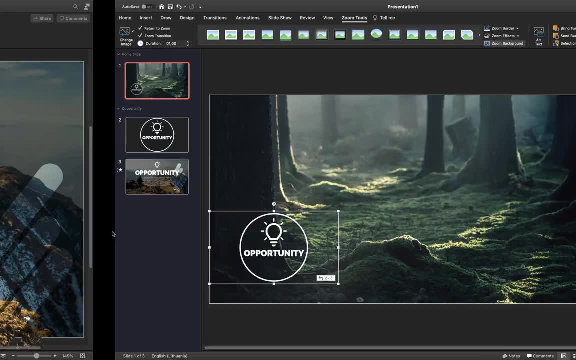 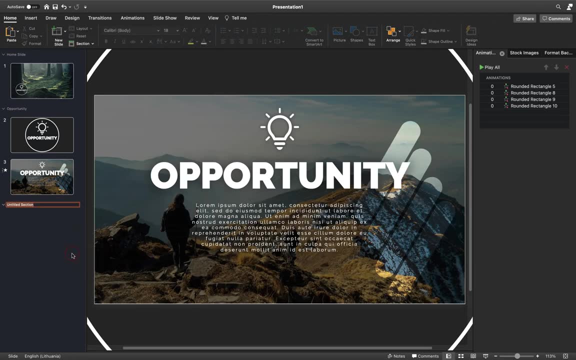 gentlemen, so we have created our first slide section, opportunity, and now we can start creating our next section, which is called market. so let's add a new section, let's call it market, and we can copy the slides from the opportunity section and let's paste them into the market section to save some time. let's make sure we keep. 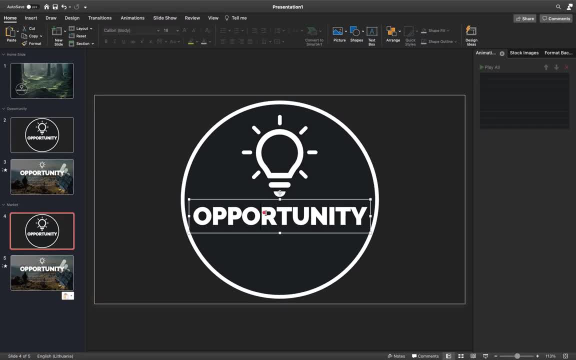 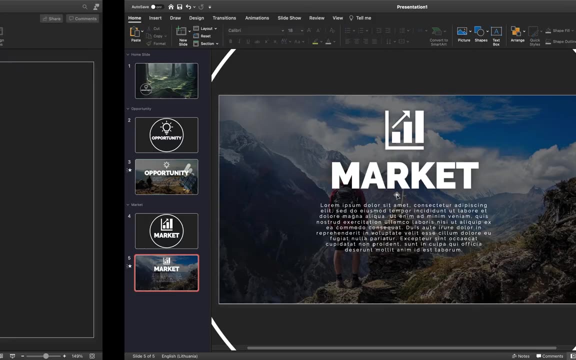 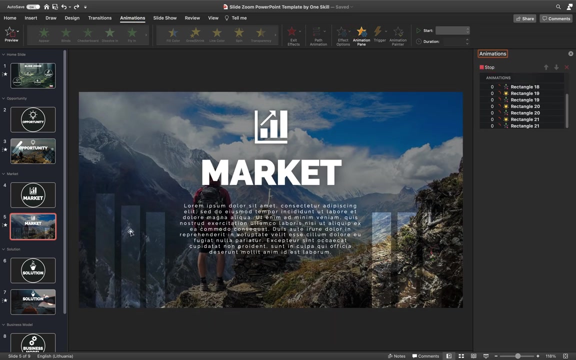 source formatting. that's beautiful, alright. so now we have to do a couple of changes. I will quickly update the text boxes, change the icons and find a new beautiful background picture. you know how we can add these animated rectangles to our market slide, which look like this: as you can see, they're growing up and down. so for that we have. 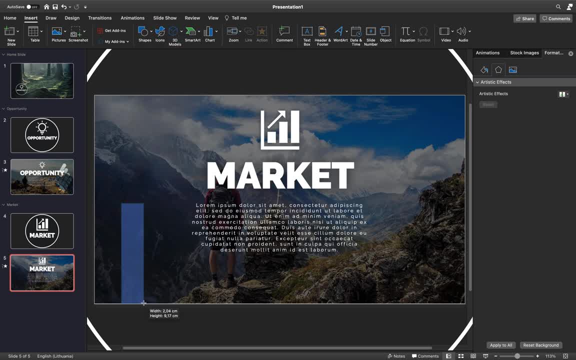 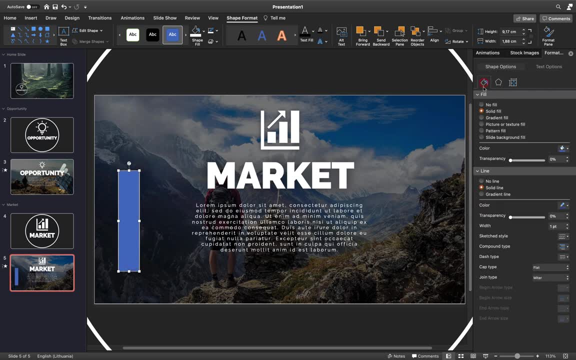 to go to insert shapes, and let's choose a rectangle, a simple rectangle, and let's make sure that we set the slide background as the fill option for our rectangle. that's awesome. and for the lines, let's choose no line. all right, and now we can start playing with. 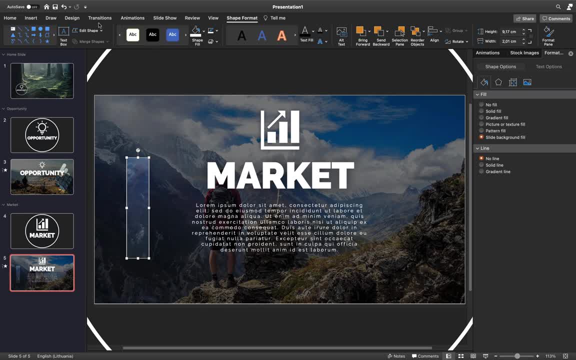 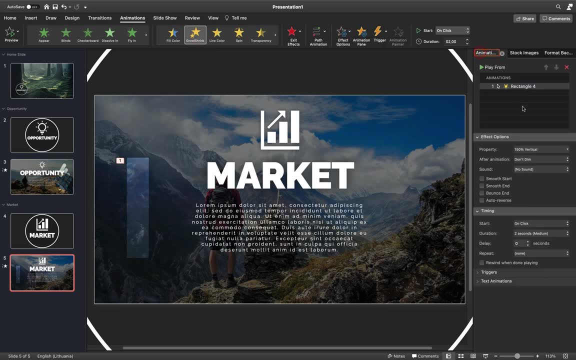 animations. so let's go to animations and let's choose grow shrink animation. let's make sure that it goes only vertically. all right, starts with previous smooth start, smooth and auto reverse, and let's set it to repeat until the end of slide. and for the growth percentage, let's choose 125 percent. you. 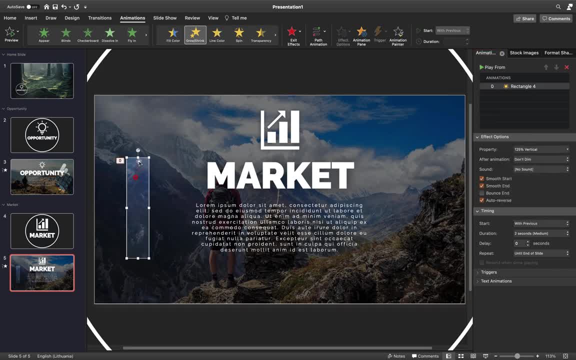 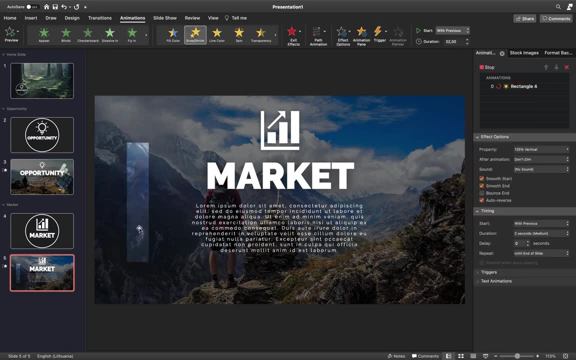 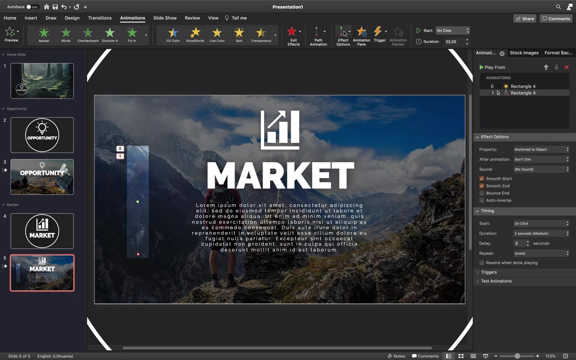 can experiment with any percentage that you would like and if we would like to play the animation right now, you can see that this rectangle is growing upwards and downwards at the same time, but we would like this rectangle to grow only upwards, so to do that, we have to add additional line animation, which goes: 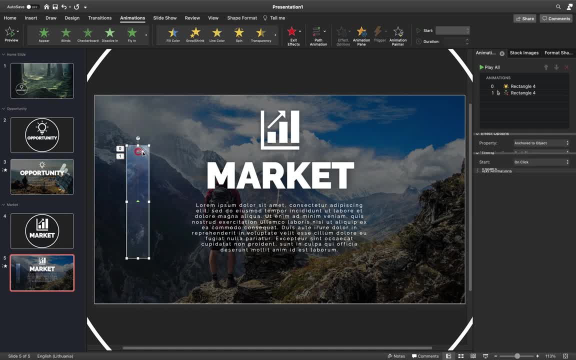 up and now we can grab and select this red bubble and adjust it a little bit so that we have only this small upward motion path and let's make sure that this motion path animation starts with previous, that it has the same smoothness- start, smooth, end- or to reverse and repeat until the end of slide. so now we can check it out and 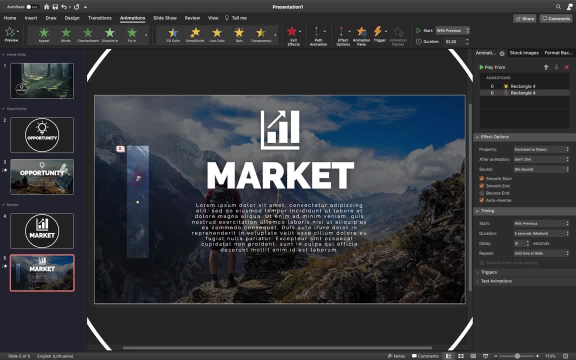 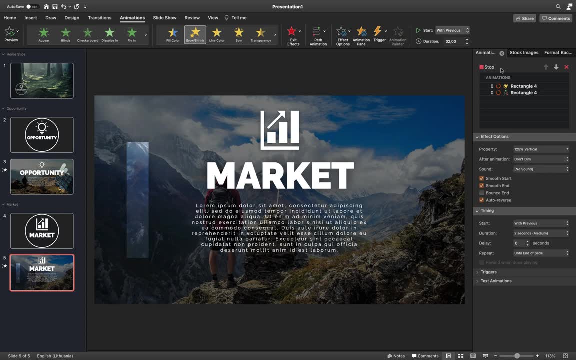 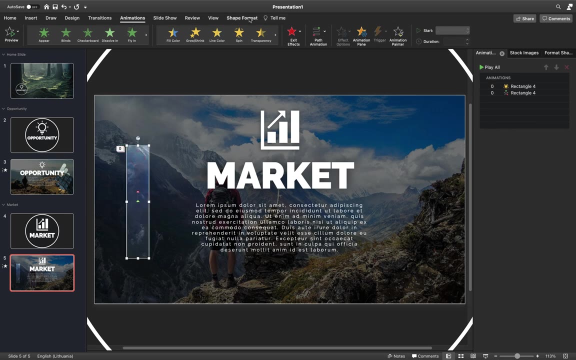 see what result do we have? so i think it's pretty close. let's reduce the motion path to something like this, and i think now it looks pretty good. it looks as if rectangle grows only upwards, so i think that's nice effect, and now let's just align this rectangle to the bottom of the slide. 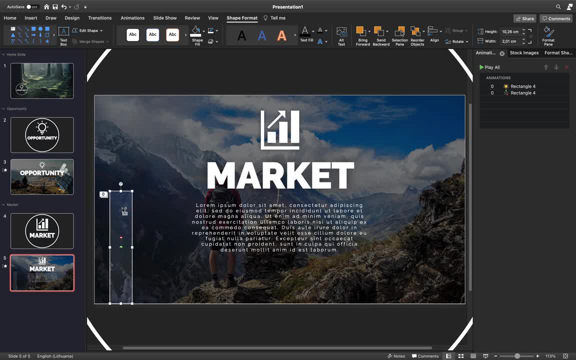 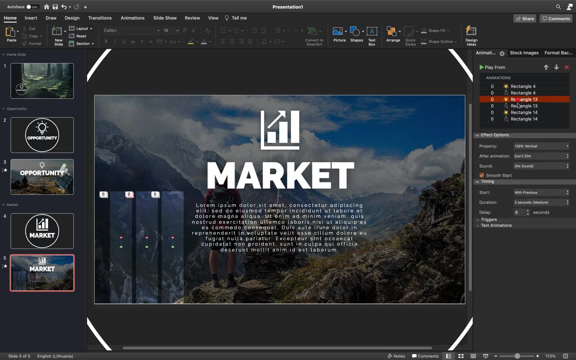 and let's make some quick copies with a option or control key and let's distribute these beautiful rectangles horizontally so that they have equal gaps. that's awesome and at the same time, let me add some delays to these rectangle animations. don't forget to add delays both to the growth shrink animation and motion path animation. all right, let's check out the. 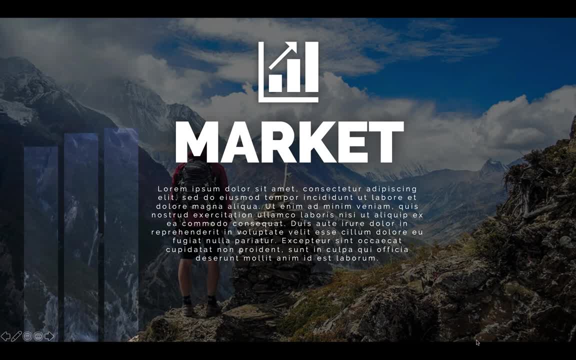 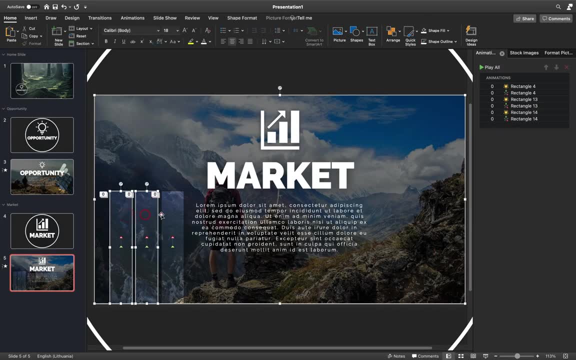 final result. as you can see, the first rectangle starts, then the second, and then the third, and we have this beautiful, fluid animation. all right, and if we want, we can select these three beautiful rectangles and copy them to the right side of the slide, so that we have six rectangles in total. let's just make sure that we adjust. 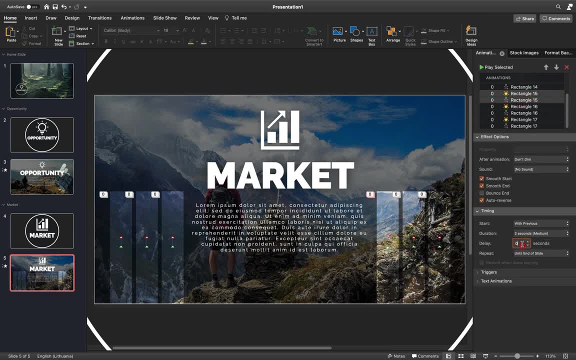 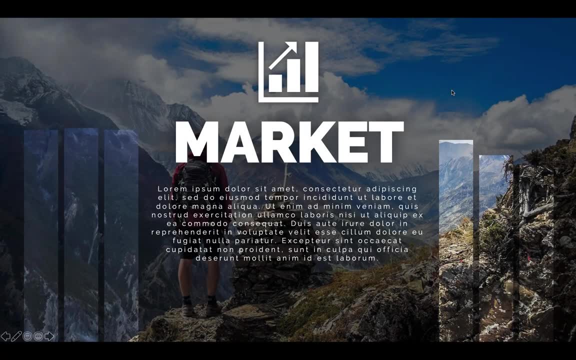 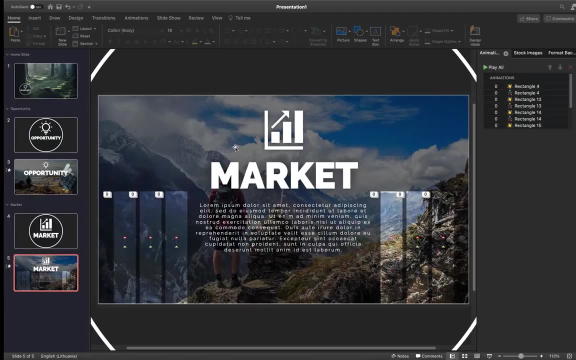 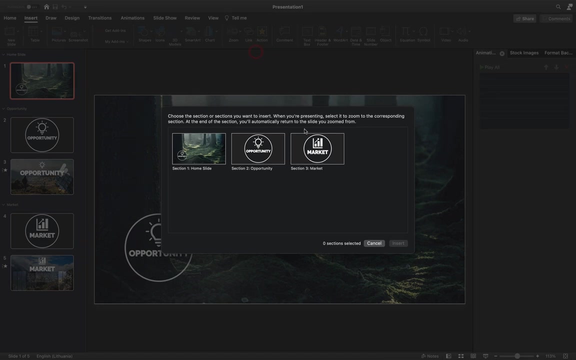 the delays for these guys on the right side and we should have some beautiful final result. skadoosh, ladies and gentlemen, this is the market slide looking beautiful. so we have finished creating two sections: the opportunity section and the market section. so now we can insert the section zoom. for the market section, let's make sure it has transparent background. that's beautiful. 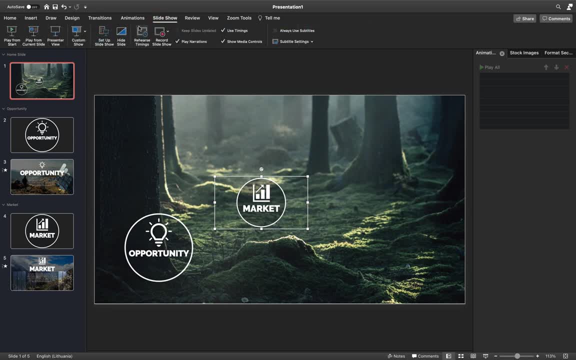 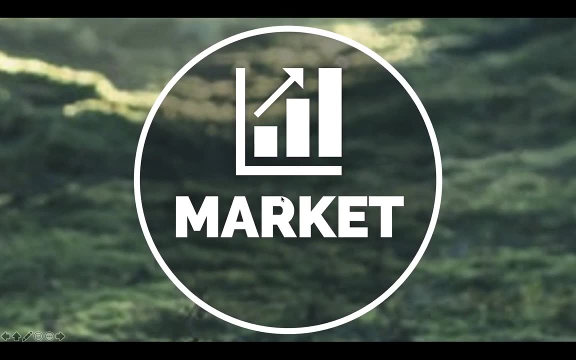 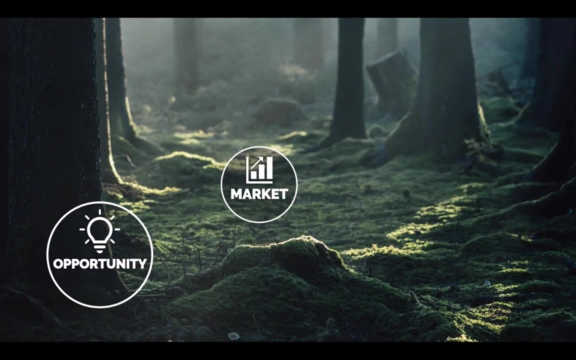 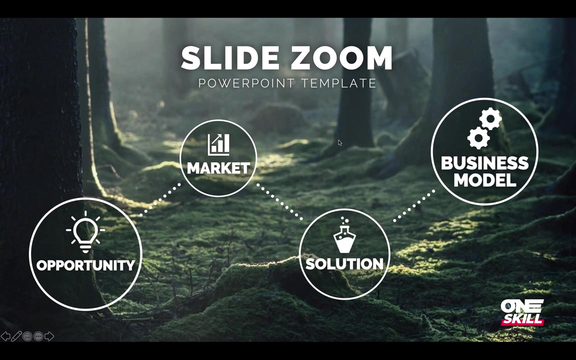 let's check it out on the full screen. if it works, should be working just fine. like I said it cinco cuatro, you should be able to see many beautiful, state-of-the-art antagonistic effects. the other reason is because the abstract angle just doesn't have enough sounds. the 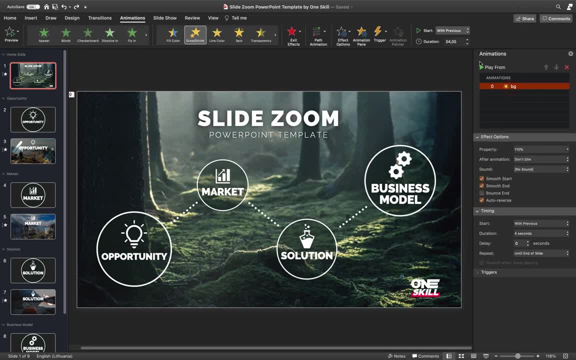 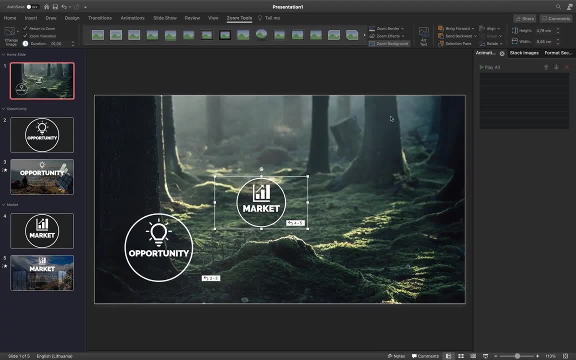 mister. but when you apply the sound dopomix to it that the turn on image onto speak not lower all we can give you surface. so let's just do some его hunting3.i use the nasadid auto reverse, so let's just copy this animation with the animation painter and paste it to our 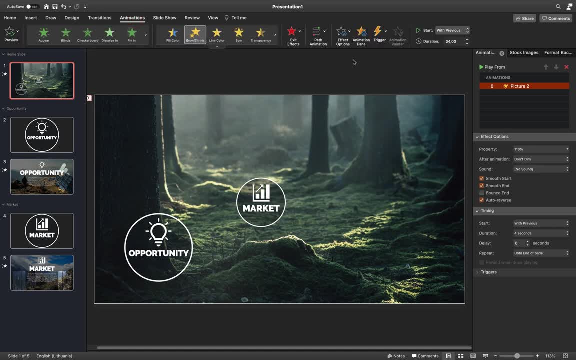 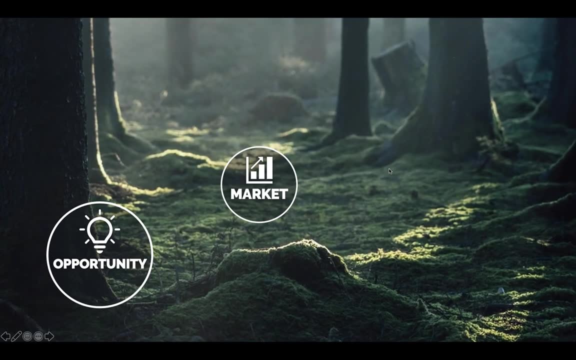 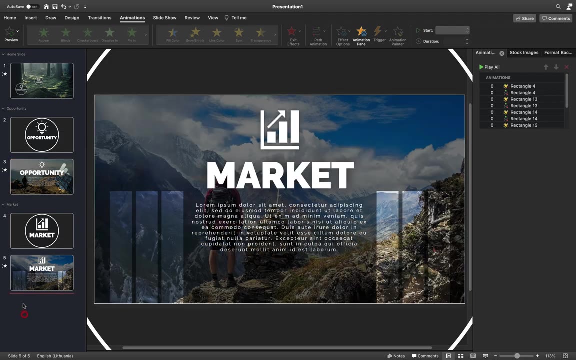 home slide 110 growth. shrink animation starts with previous. all right, and this is how it looks like on the full screen. that's beautiful. all right, ladies and gentlemen. so let's continue with the next section, which is, as far as i remember, solution. all right, so let's add a new section. 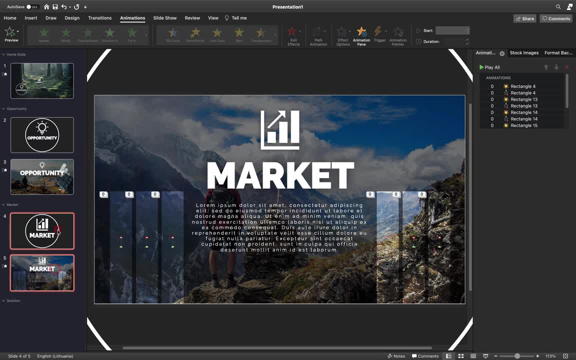 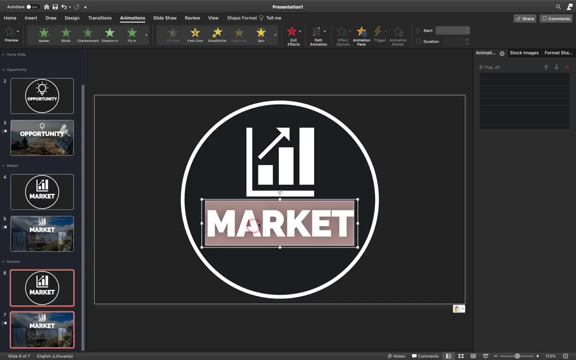 let's call it solution. let's copy these two slides from our previous section. let's paste them right here. make sure we keep the source formatting and, as before, i will speed up a little bit and do some updating for the text boxes, icons, and i will find a new slide background picture. 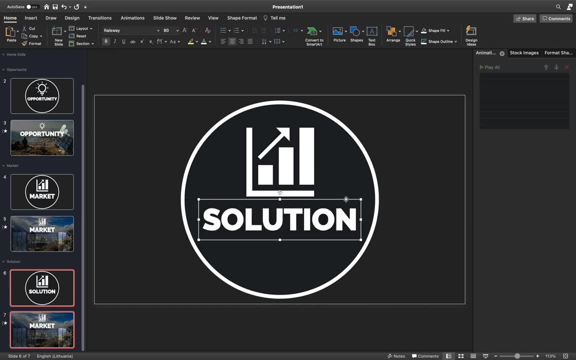 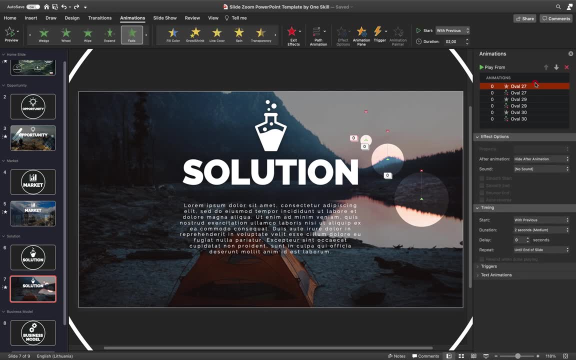 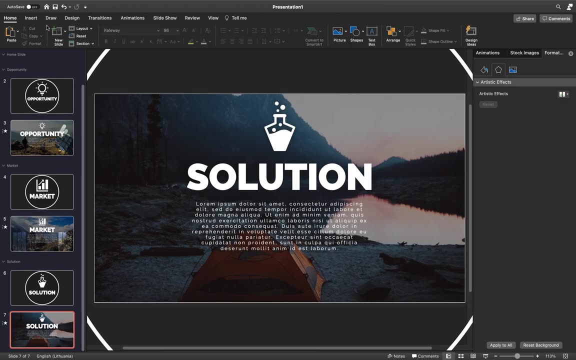 and i'll meet you when we will be animating some awesome bubbles. so meet you there. all right, so let me show you how we can create these animated bubbles here on the right side of the slide. so let's get back to our presentation, go to insert shapes and 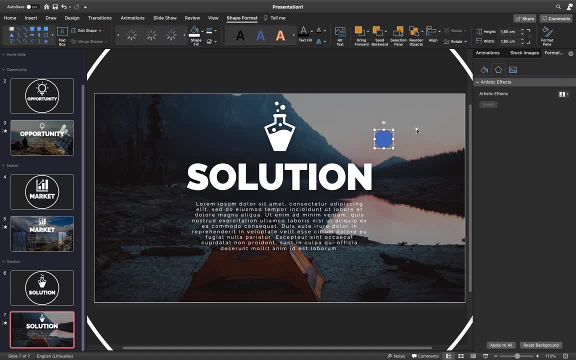 choose the circle tool. hold down the shift key to get perfect circle and once again, let's set its fill to slide background and no outline. that's awesome. now let's go to animation and let's choose line animation. let's make sure it goes up. adjust the red bubble to 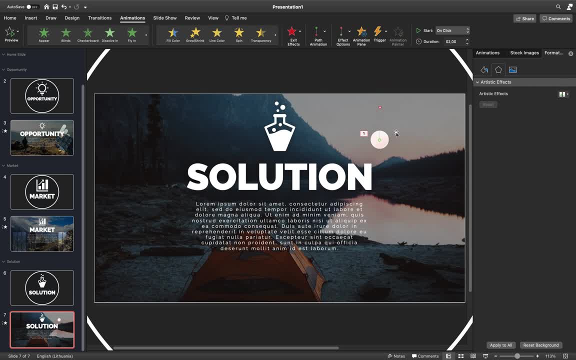 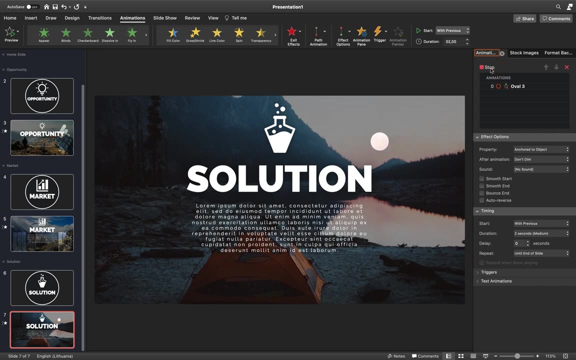 adjust the distance to something like this: all right, let's make sure it starts with previous: no smooth start, no smooth end, just repeat until the end of slide. so this is how the animation looks like. all right, and let's add a second animation, which is fade, and. 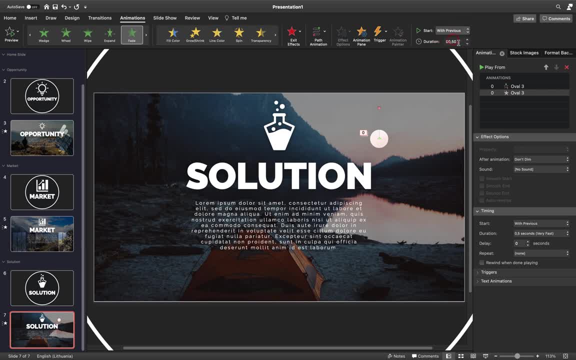 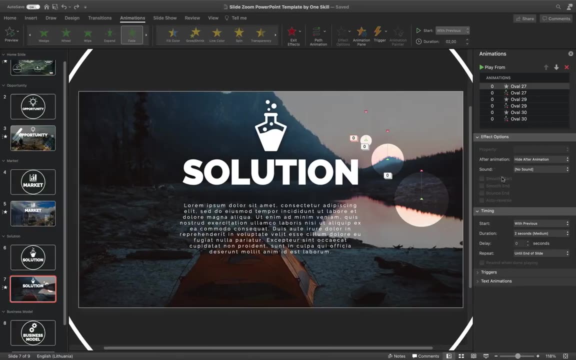 animation to the same circle. let's make sure it starts with previous, the same duration- two seconds- and repeats until the end of slide. so this is how the final result should be looking like. so the bubble goes up, it pops and it repeats, so now we can quickly copy this. 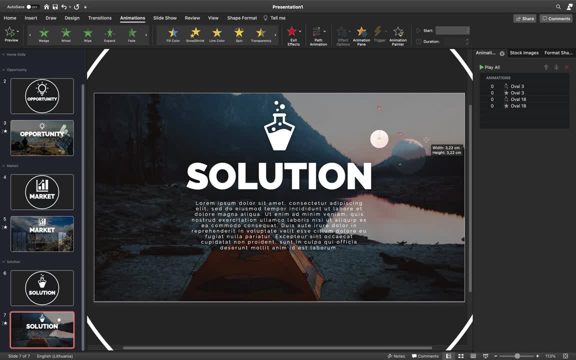 bubble. a couple of times we can increase the size of the copies to make it more interesting, and after that i'll just add a little bit of delays for the second bubble and for the third bubble, so that we would have a little bit more interesting looking animation. 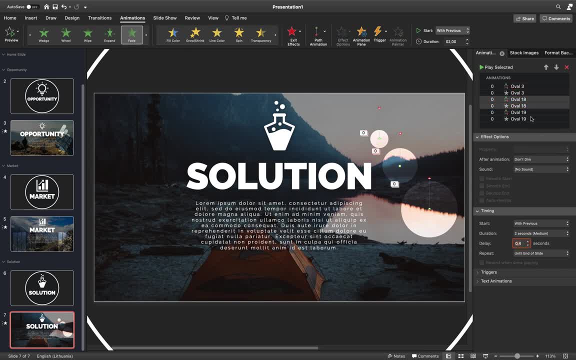 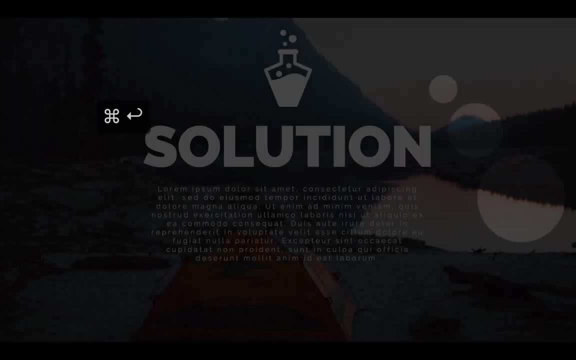 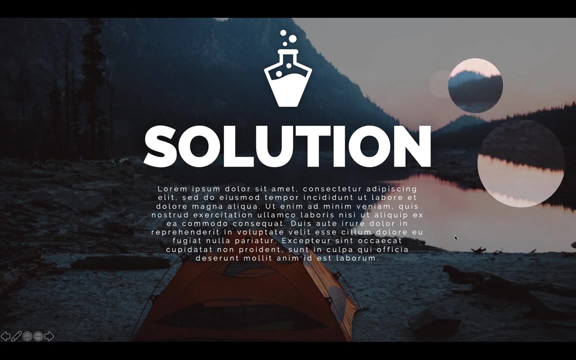 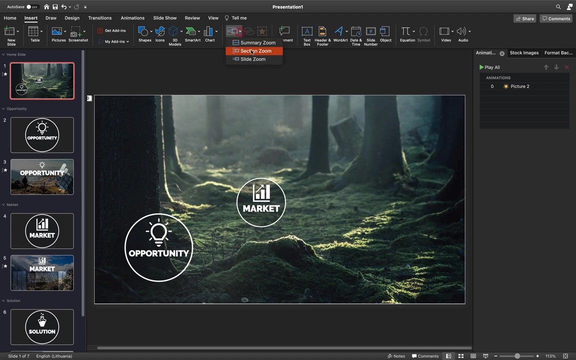 so for the second bubble, 0.4 second delay, and for the third bubble, 0.8 second delay. and this is the final result looking beautiful, all right. so the third section is completed. so now we can insert section zoom in our home slide. let's choose solution section. let's make sure it has transparent background. 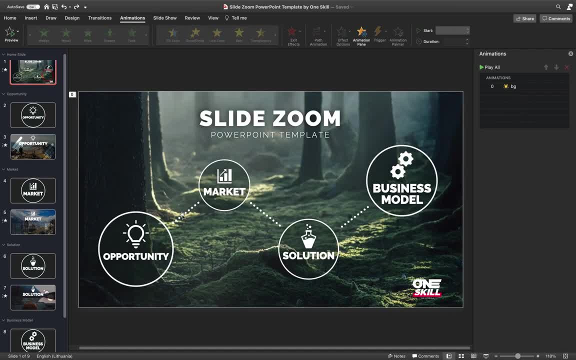 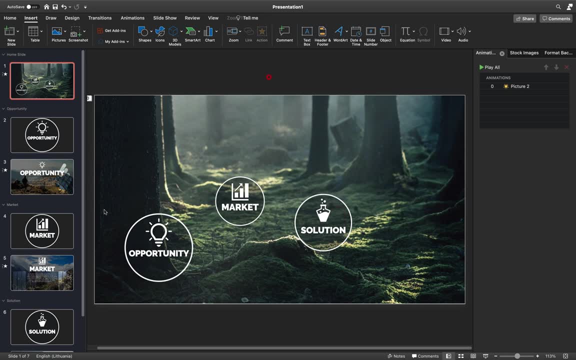 we can increase the size of the section zoom if we want and, by the way, as you can see, we have these dotted lines. i'll show you how we can create those lines a little bit later, later on. and now let's continue with our last section, which is called business model. 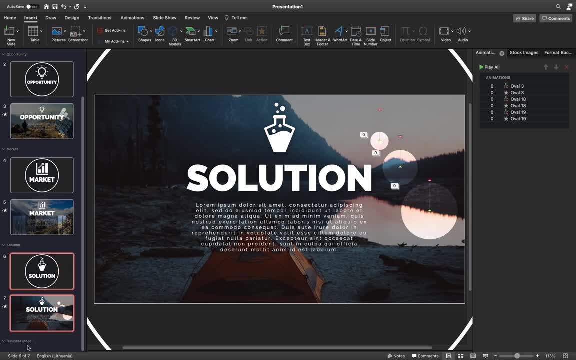 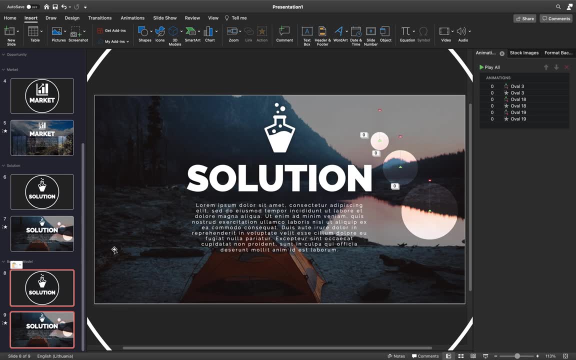 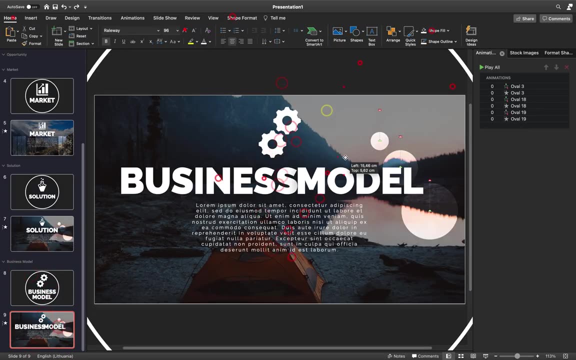 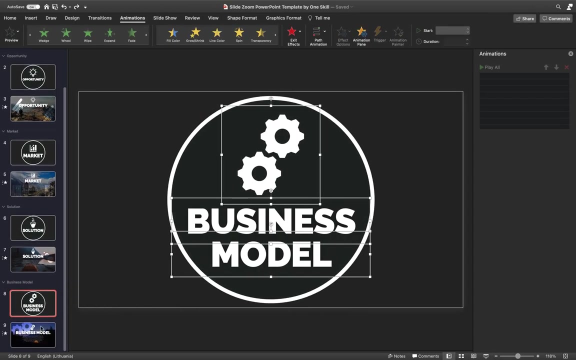 and, as before, let me copy a couple of slides from any previous section and let me do some updates. so i will change the text box to business model, change the icon and find a new beautiful background. all right, so let me show you how we can create this beautiful spinning gear animation for our 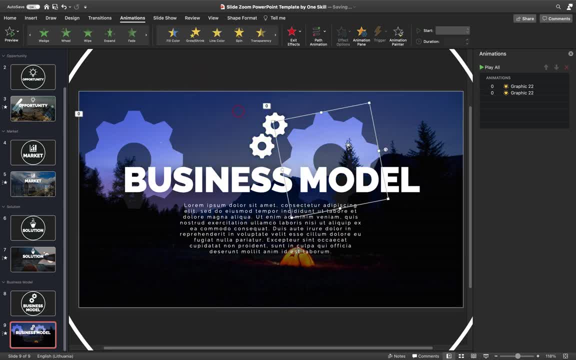 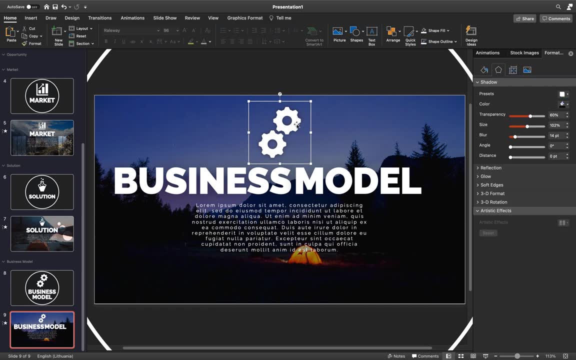 last slide so you can see we have some gears and their fill is set to a background fill. that's super, duper awesome. so first i thought that i could easily, you know, subtract one of these gears from this gear icon. so that's what i did. i now made a copy of these gears. then i have. 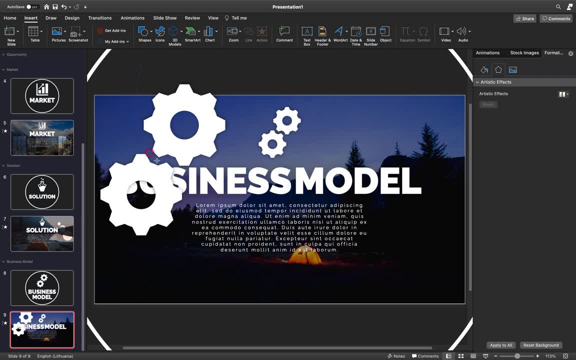 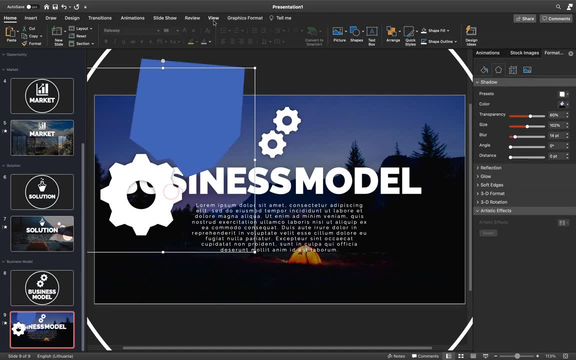 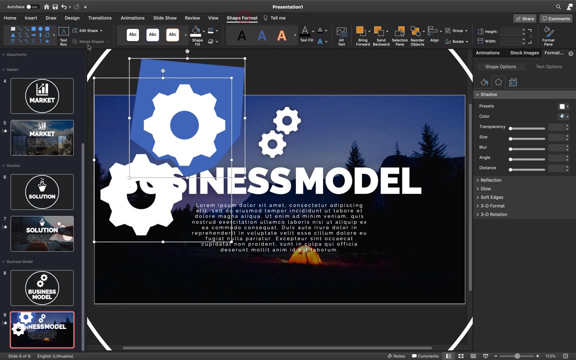 inserted a free form shape so that i would cover one of the gears. all right, so here's the shape and let's convert our gear icon to shape. all right, so let's select the gear shape, hold down the shift key, select the blue shape and, as you can see, the merge shape function is not available. so how can we actually cut one of? 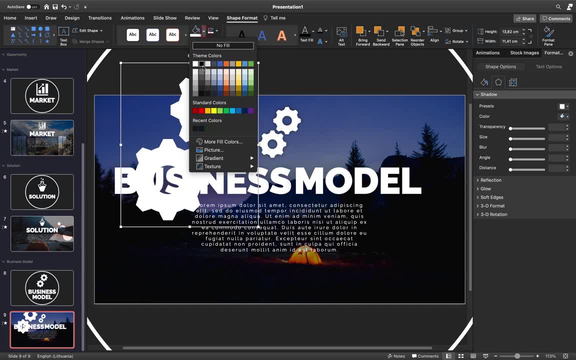 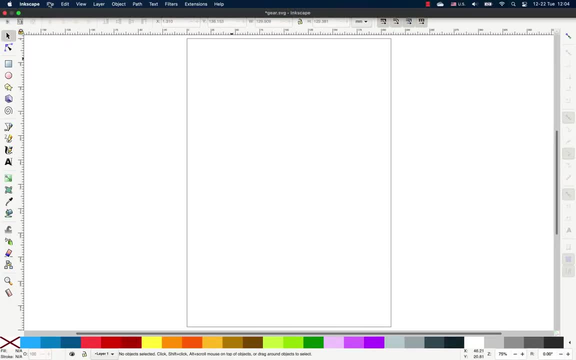 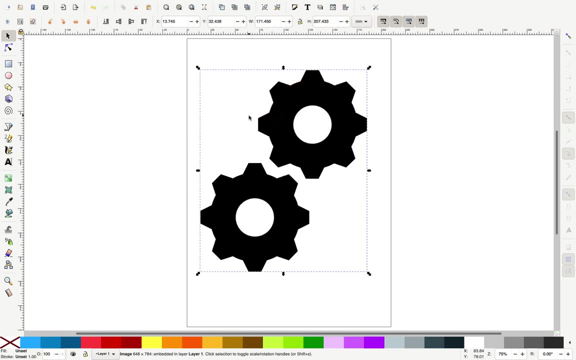 the gears off. so first let's just make them black, and now let's just cut these gears and let's go to a free, open source vector program, all right, so let's paste those gears right here. now they are just as a picture, so let's select it and let's go to path and choose trace bitmap, which will 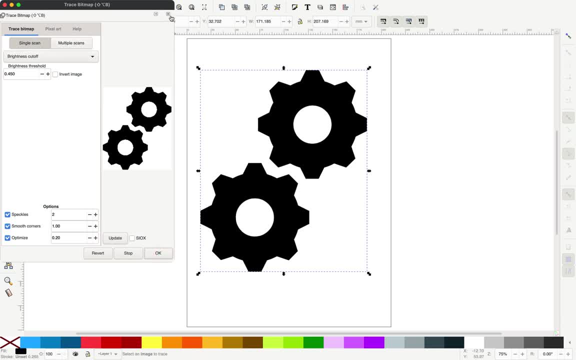 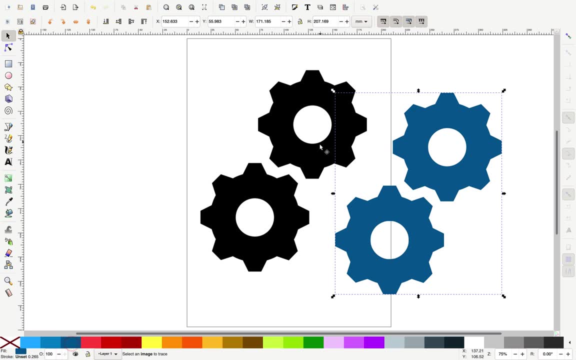 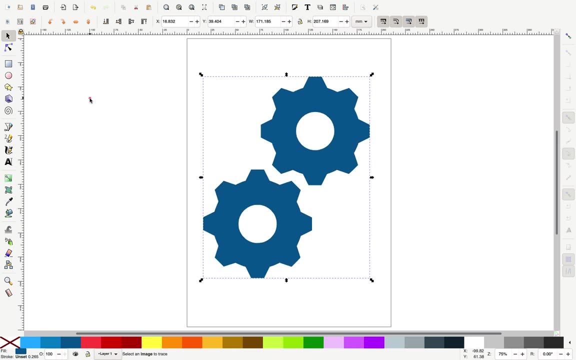 basically help us to make a vector copy of these gears. so let's just hit ok. so now we have a vector copy. we can change the color. that's awesome. and for this picture we can delete it, okie dokie. and now let's just use this tool to create a free form shape, just the way we did in powerpoint. 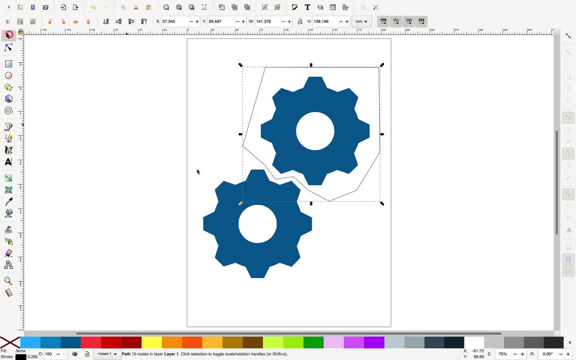 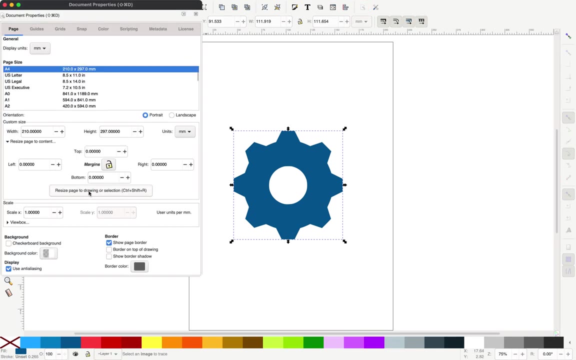 except this time it will work. so now we can select our gears, our free form, shape. and now let's just go to path and choose difference. so it's pretty much the same as subtract and powerpoint. all right, so we can just resize the whole document to the size of this gear. that's awesome. and now we 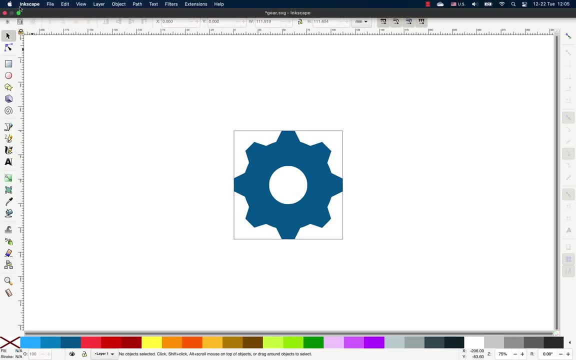 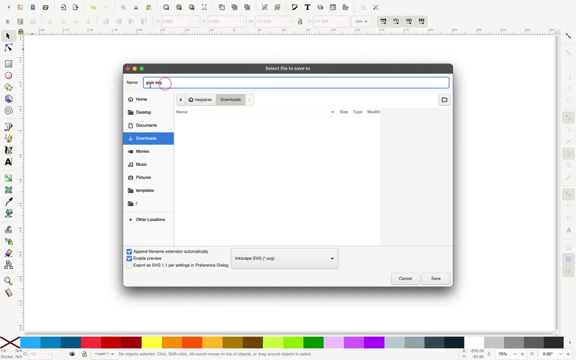 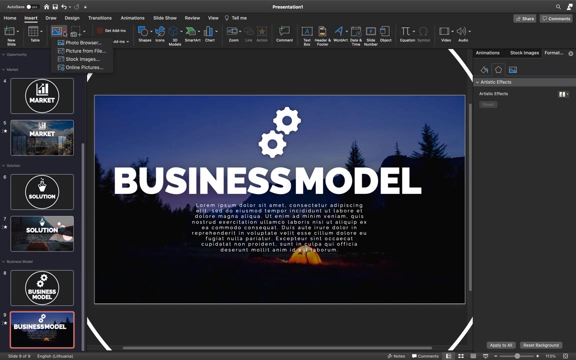 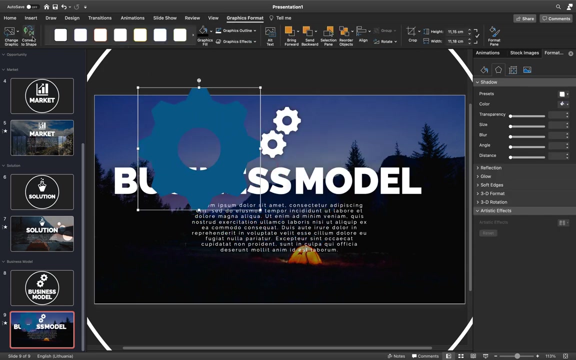 can export this gear as an svg file. so let's just save it as svg file. that's super duper awesome. and now we will be able to import this gear into powerpoint as an editable shape. so let's just go to pictures. choose our gear svg. that's awesome. let's click convert to. 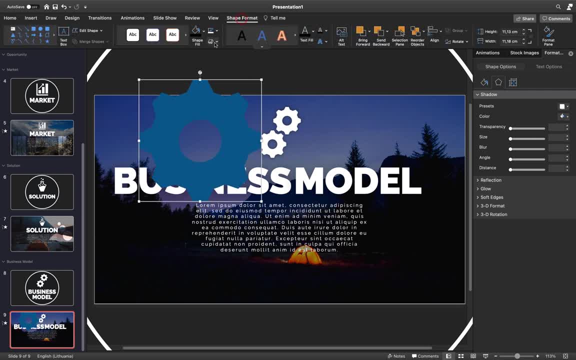 shape. so now it's an editable shape. we can change its color. and now if we would copy this gear? let's make a second copy. select both of these copies. now, as you can see, the merge shape functions are visible. so that's pretty awesome. but, as you remember, we 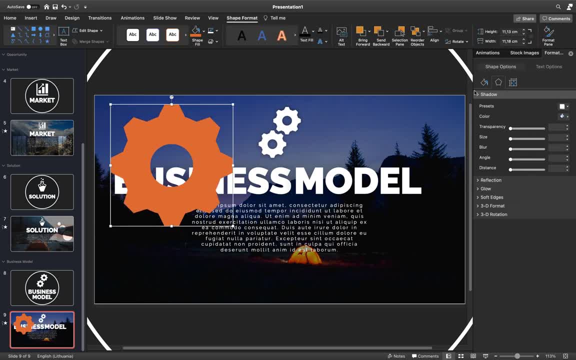 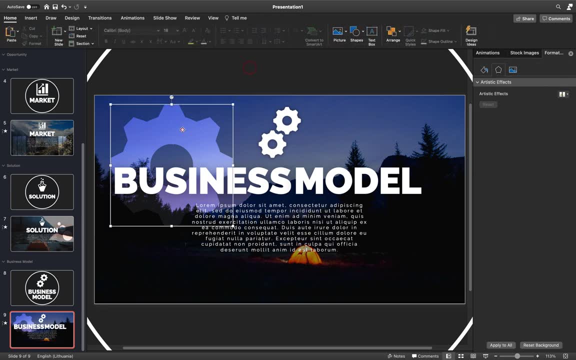 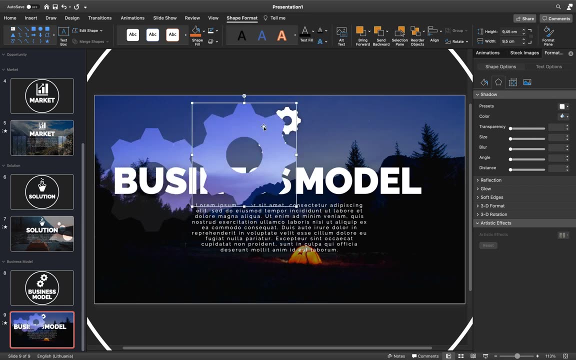 have to set the fill of this gear to slide background. so let's just go to fill options and choose slide background fill and let's just make sure that text box is on top. all right, let's reduce the size of this gear and now we can start working with animations. let's make 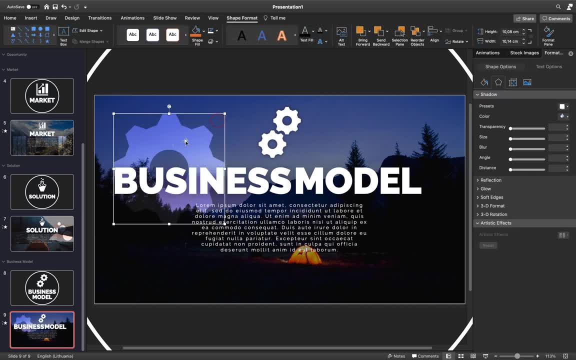 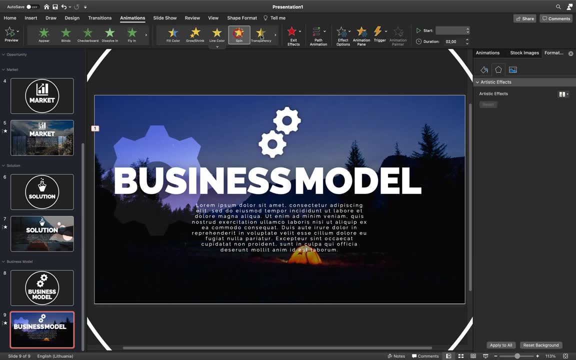 sure that there's enough place for the second gear. a few more adjustments, all right. and now in the animation spin, let's choose spin animation. okay, let's make sure it starts with previous duration, something about seven seconds. let's make sure it goes clockwise, makes full spin and it repeats until the end of slide. 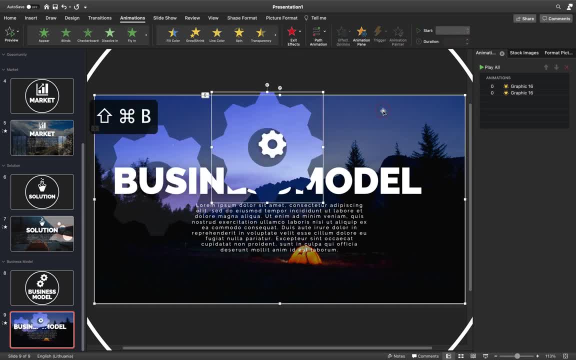 all, right now we can quickly copy with the option on the original animation. it's actually a little bit tricky, so it's just a good idea to do the same thing and that's it. so let's not do it too quickly, let's focus on immediately in the animation. 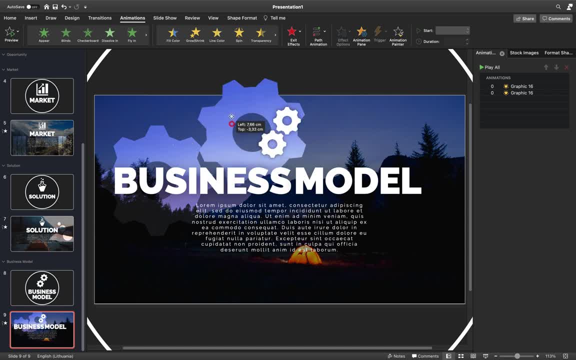 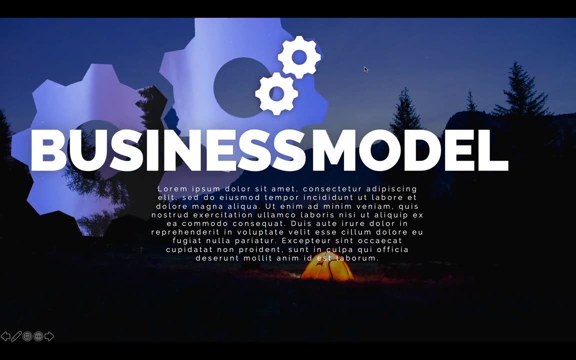 we were doing by using the tool, key this gear and now let's position it so that you know these uh gears nicely connect to each other. and for the second gear in the animations, let's make sure that the spin is going anti-clockwise or counter-clockwise, i guess, yeah. 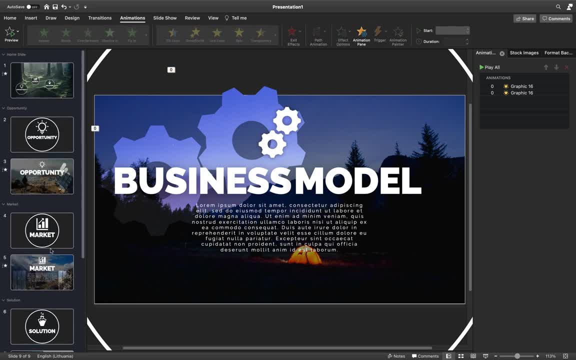 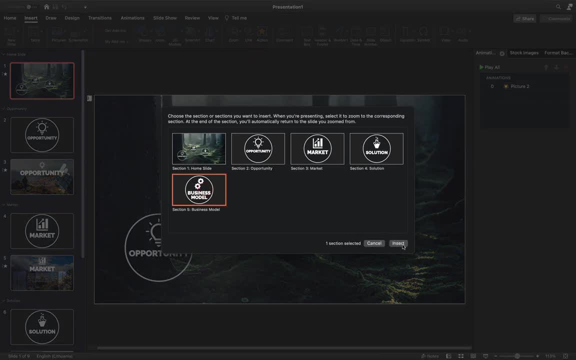 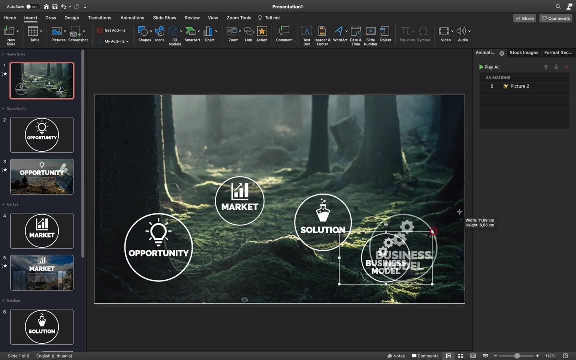 counterclockwise our last section, so we can insert a section zoom in our home slide. so let's just go to zoom, section zoom, and let's find business model section, hit insert. make sure that our background is transparent, all right, and now we can adjust size and position of all of these section zooms until we get the 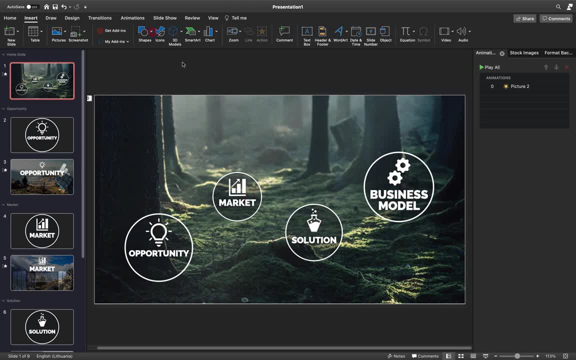 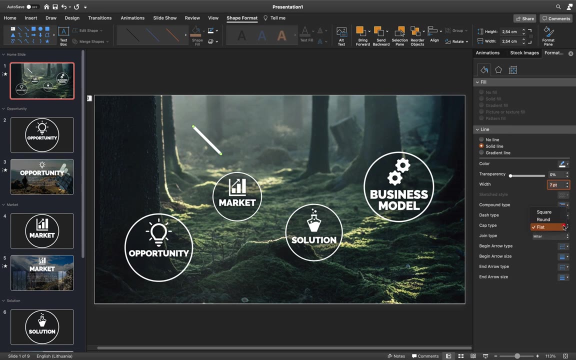 look that we want, all right. and now let's connect these. section zooms for the beautiful dashed line. so let's just insert a line which is blue. so let's make it white so that we can see it. all right, and in the width options let's give it a width of seven points. let's make sure that the cap and join. 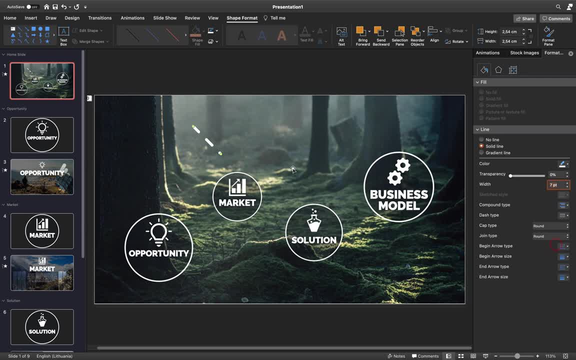 is round, all right, and for the dashed options, we can choose any dashed style that we want. all right now we can use this line to connect all of our section zooms and, as before, you can quickly copy any object while holding down the option or control key. my friend, and if you'd like to choose a different, 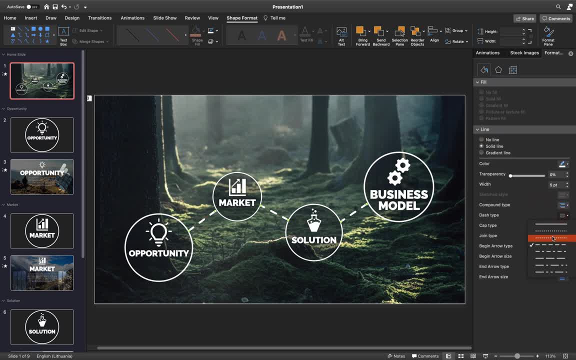 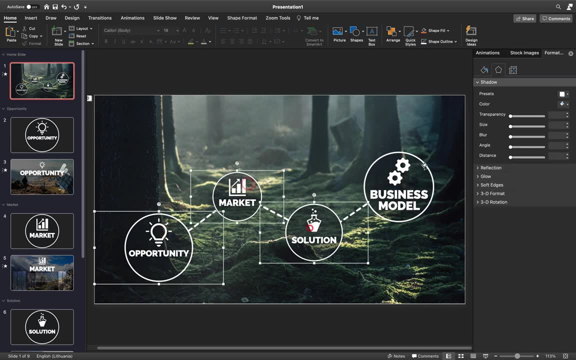 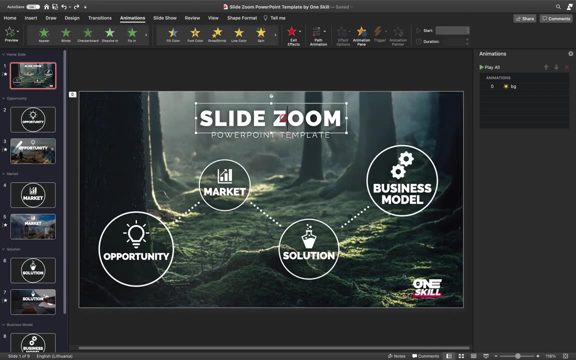 dashed style. you can select all of your lines and choose a different style. for example, this one looks awesome. all right, and we are pretty much finished and let's just make sure that we bring all of these section zooms to front. and let me copy the title and subtitle and one skill logo. 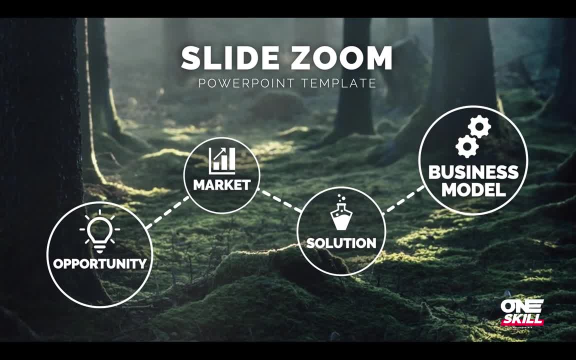 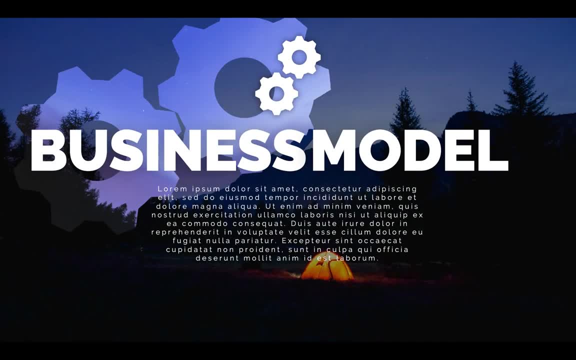 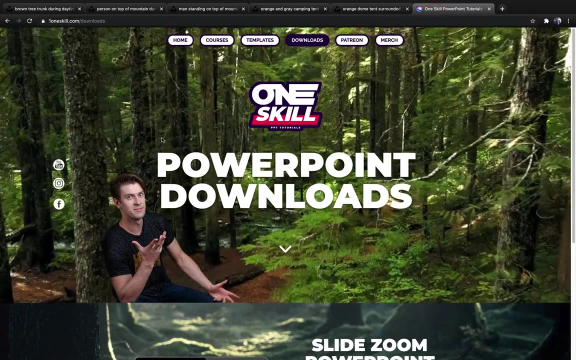 and we'll see you in the next part of this video. thanks, ladies and gentlemen, we are finally finished. now you know how you can create this awesome slide zoom powerpoint template with clickable section, zooms and awesome animations. and if you'd like to get this slide zoom powerpoint template for absolutely free, just go. 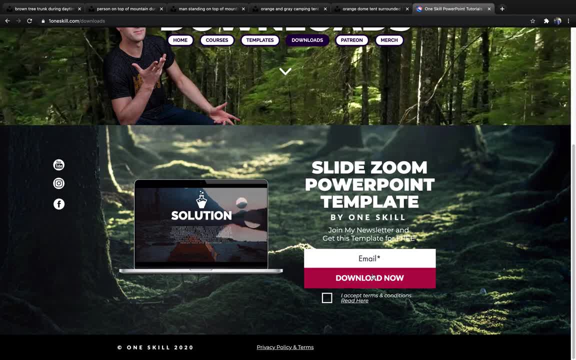 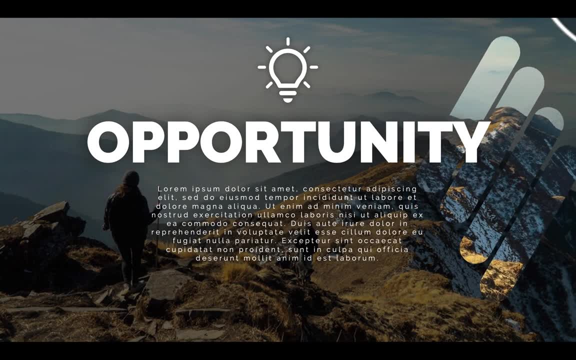 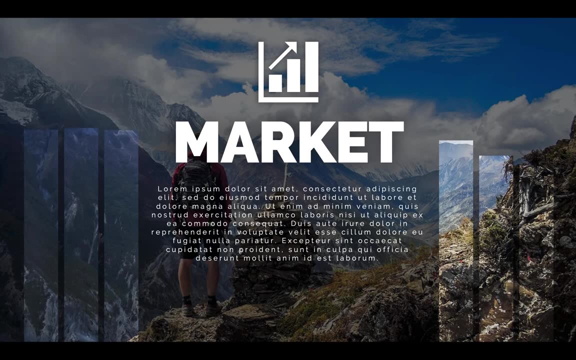 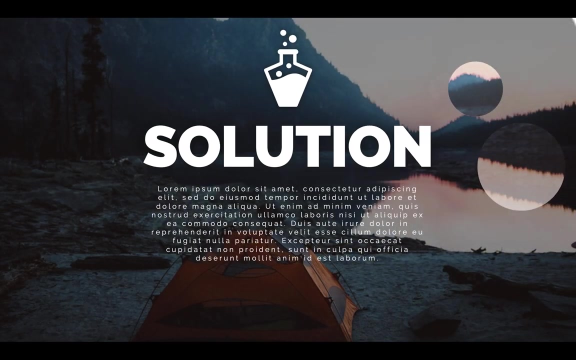 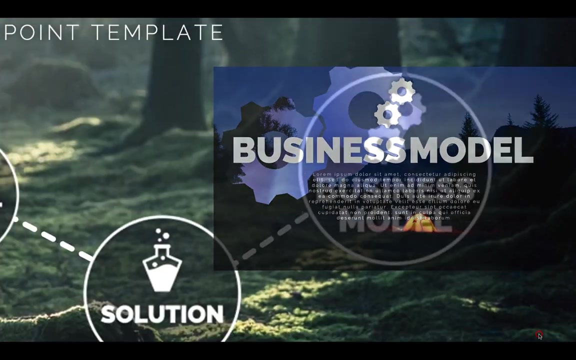 to my website download section, insert your email and i will send you this awesome template right away. so, ladies and gentlemen, thank you for watching, stay happy, stay healthy and i'll see you in the next part of this video or my next video. you.